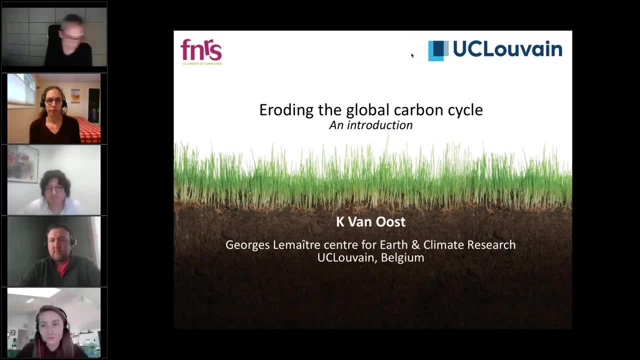 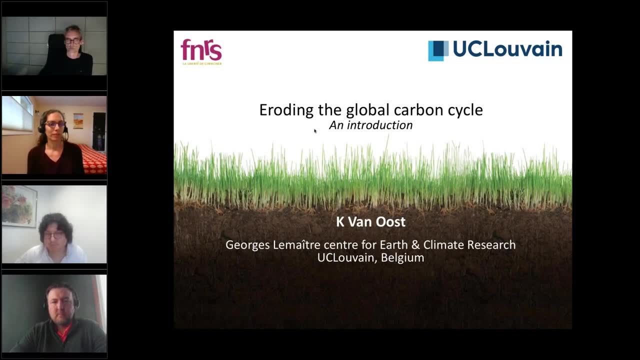 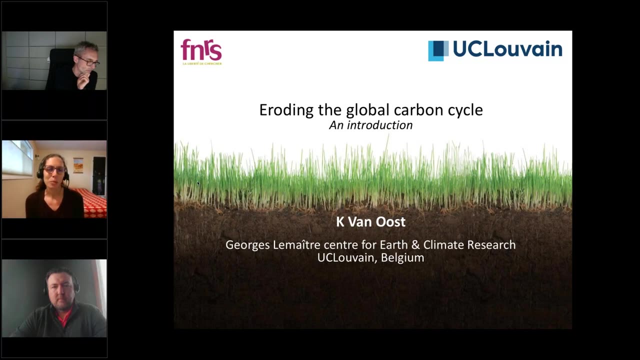 Hello and welcome to our first ISCN webinar of 2022. And as folks are filing in, I just want to let you know you are in the right place if you're here to learn about impacts of soil erosion on the carbon cycle and on carbon sequestration. 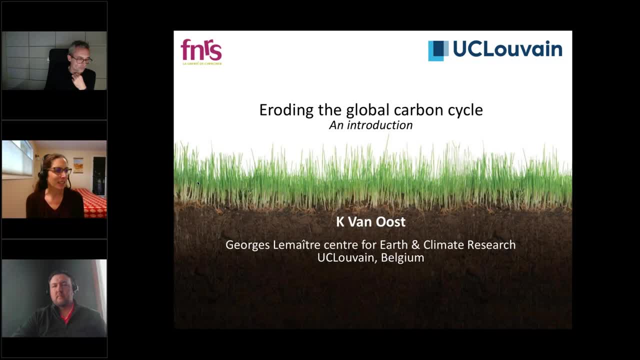 We have about 270 people registered for the meeting, so it'll take a couple minutes for everybody to get into the virtual room. But I'll let you know that we have two wonderful speakers with us today. We have Christophe van Oost who, we're so fortunate, is willing. 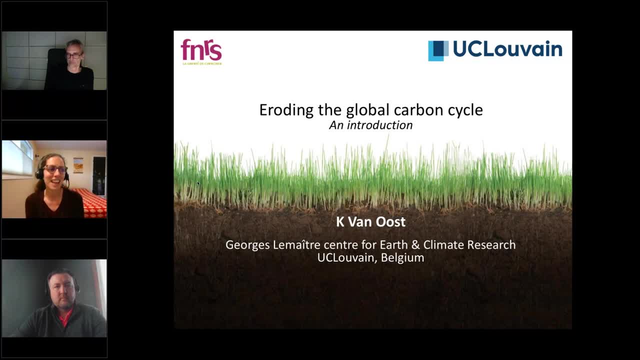 to call in from Belgium, where I think it's nine o'clock at night, And he's really a leading expert on this topic and will be able to give us a global perspective on soil erosion and carbon. And then our second speaker is Ken Wakka, who's a soil scientist and erosion. 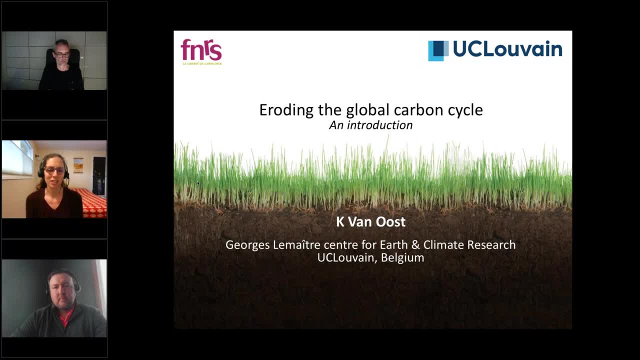 expert associated with the National oh gosh National Soil Erosion Laboratory in Indiana, So he'll give us more of a field of catchment, scale perspective and within the Corn Belt as well. So I want to give these speakers as much time as possible to give their presentations. 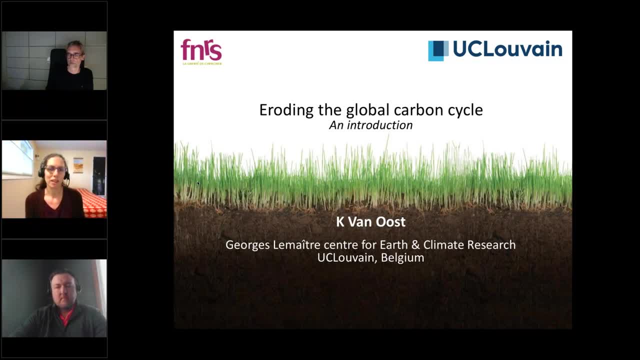 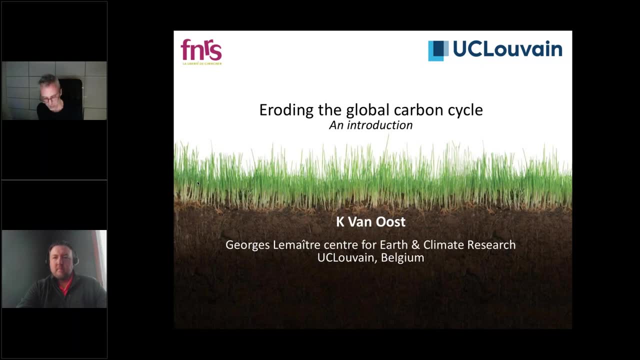 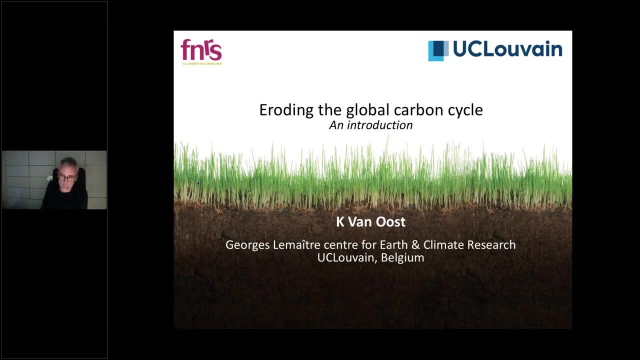 So, Christoph, when you're ready, please go ahead. Okay, thank you so much for the introduction and also thank you for the invitation. It's a nice opportunity to share a bit of my research to you guys there in the US. I would like to talk a bit about my research I did on erosion and the links with the carbon. 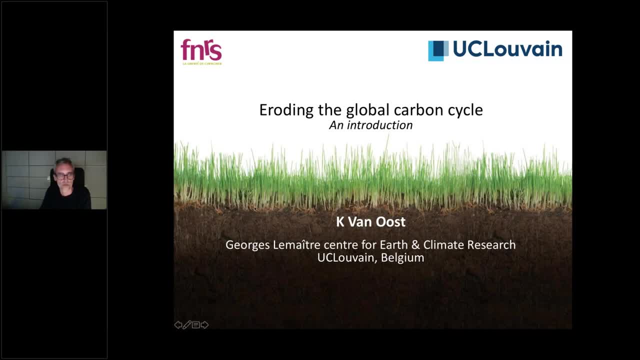 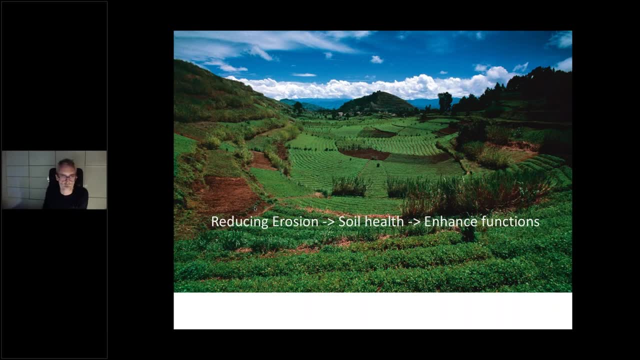 cycle. I'm just trying to get my slides correct. Yes, So I think we all know that erosion is one of the biggest threats for soil health, And it also implies, of course, that with erosion by soil conservation, there's a lot. 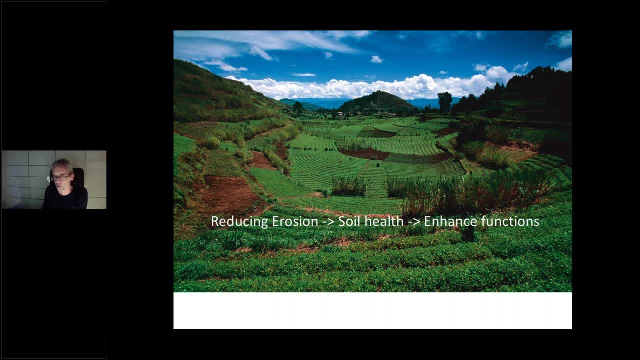 of risk And management is, of course, critical to enhance soil functions, And one of those soil functions is, of course, soil carbon sequestration, which is directly related to our climate, And this is actually the topic I would like to address today. 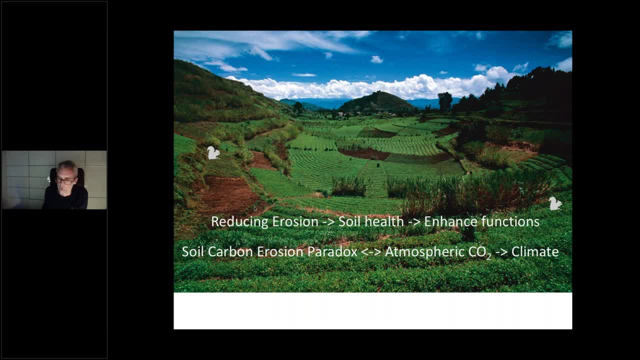 So at present there is a bit of a controversy in the scientific literature whether agricultural soil erosion actually represents a sink or a source for atmospheric CO2. And which has, of course, big implications for understanding of climate change, both past, present and future, of course. 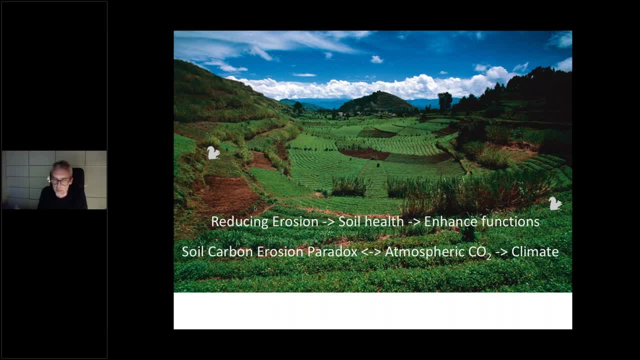 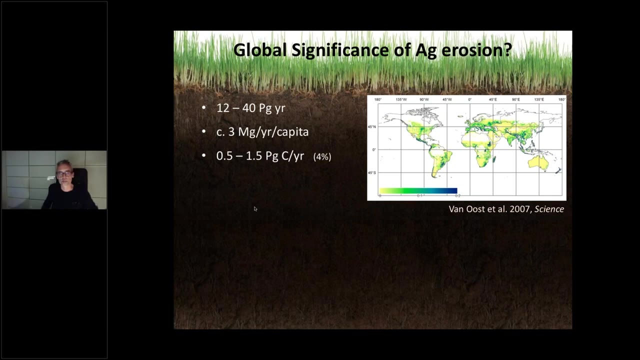 And so this is the topic that I would like to address And, as already introduced by Claire, I will do this a bit from a global perspective and talk a bit about the underlying processes. Before I start, I would like to briefly go through the 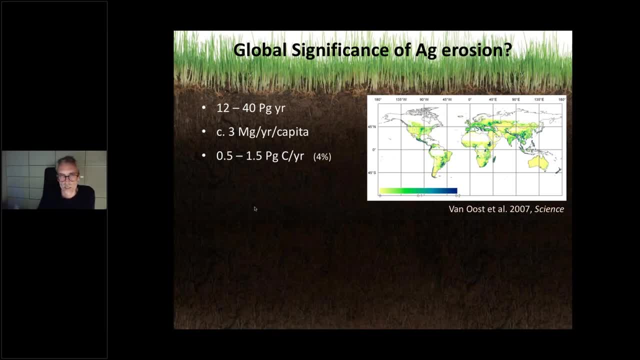 The global significance of agricultural erosion as if you go to literature there are many estimates available. Of course there's quite a big uncertainty on how important human-induced so agriculture erosion actually is. but the main estimates kind of range between 12 and 40 petagrams. 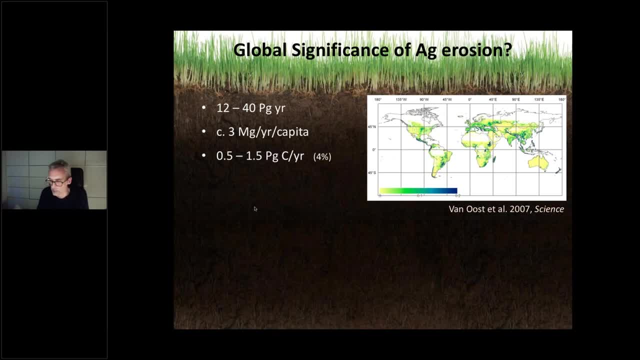 per year, And I know this number is not very meaningful to you, So I try to pinpoint that in a better way so you can also think of it. in order to produce your food on basis, we have to erode about three megagrams, which is one. 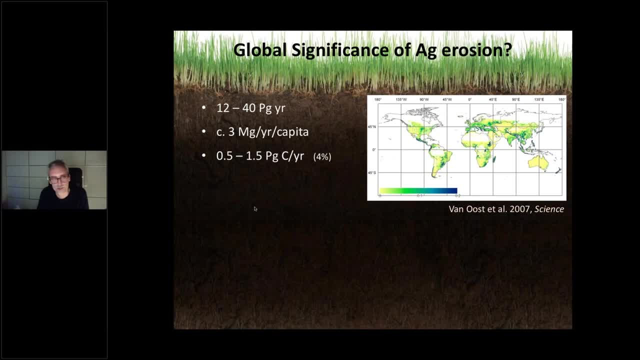 So one megagram is one metric ton. I don't know the American units, my apologies. So it's about three tons per year that you basically erode from our fields to produce your food. Okay, Okay. So I think we should be done. 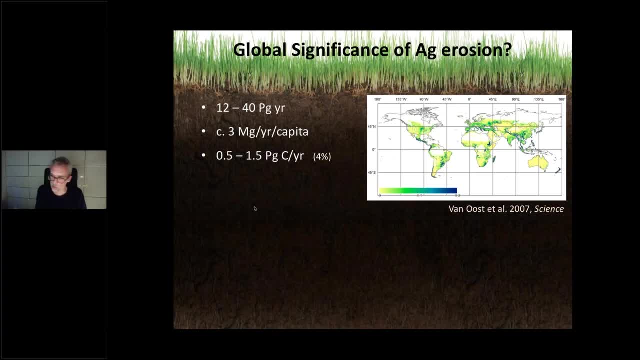 So we erode our soils, but of course they're so organic carbon, which is associated with the soil particles. If we connect that to carbon content of the eroded soil, you basically end up with an estimate that annually- every year- about 0.5 to 1.5 petagrams of carbon are being lost. 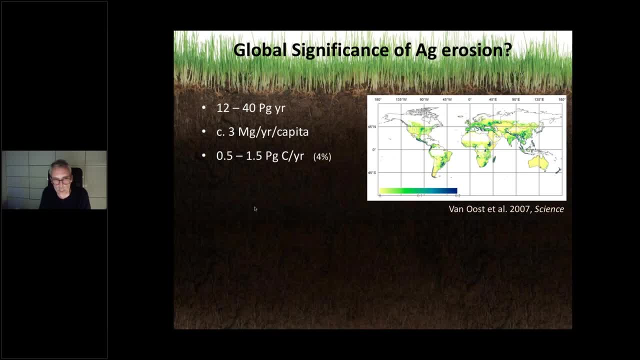 from our fields to reproduce our food. Again, this number might not be very meaningful to you, So I try to frame that a bit. So that's about four to 5% of the annual emissions in relation to the combustion of fossil fuels. 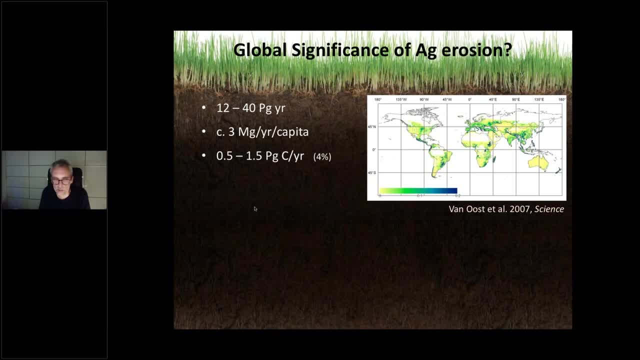 And so that's quite significant. that's a large percentage of that significant one. As you can see on the map on the right, it's not a uniform pattern that you will see of soil erosion on a global scale. You will clearly see hotspots. 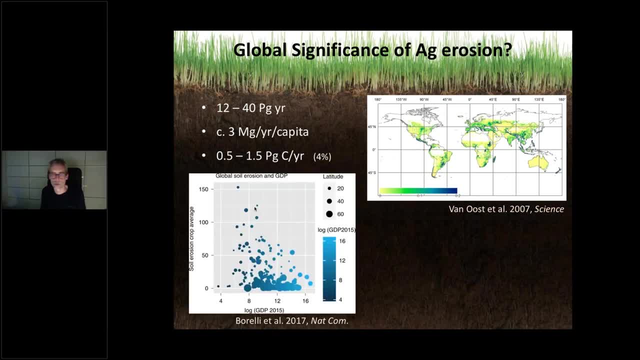 Okay, Okay. So what I would like to mention here, if you look on the graph on the left bottom side, is also the inequality which is associated with agricultural soil erosion And so on this graph, you see on the X-axis a metric for the richness of countries represented. 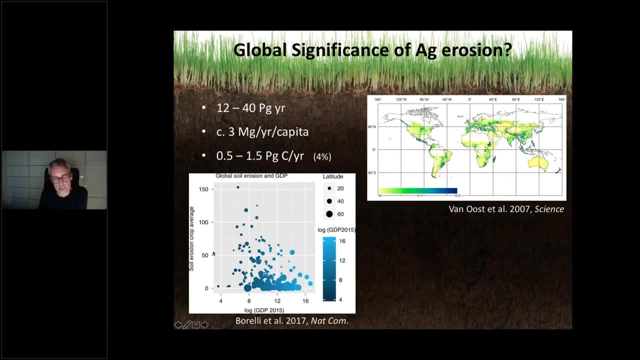 by the GDP, while on the Y-axis you see the rate of erosion, And so you can see from the color. the lighter colors are the richer countries and you see they tend to plot on the lower end, The lower end of the average soil erosion rate for a country, while the poorest countries 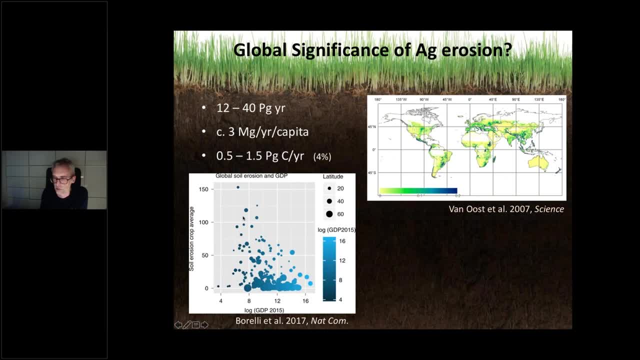 they tend also to be subjected to the highest rates of soil erosion, And of course, this is related to the fact that in the developed world we have better ways to implement soil conservation and soil management, but it's also related to the fact that most of the erosion actually occurs in the tropical regions. 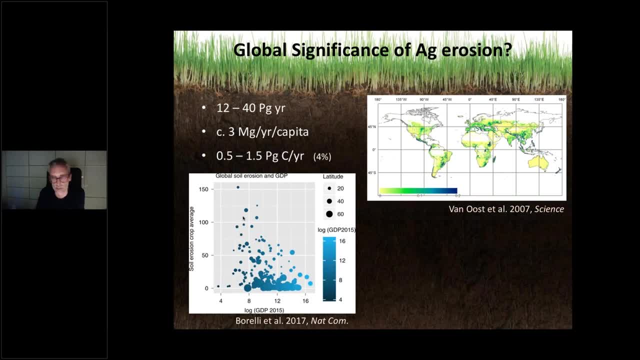 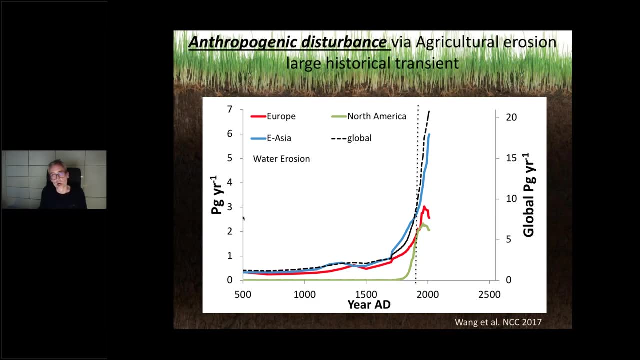 And that's why, Okay, And that's why you have this inequality. What is also interesting to see is that there is actually a very large historical transient of sediment being generated by agricultural erosion. So from the start of agriculture, this has been always relatively small. 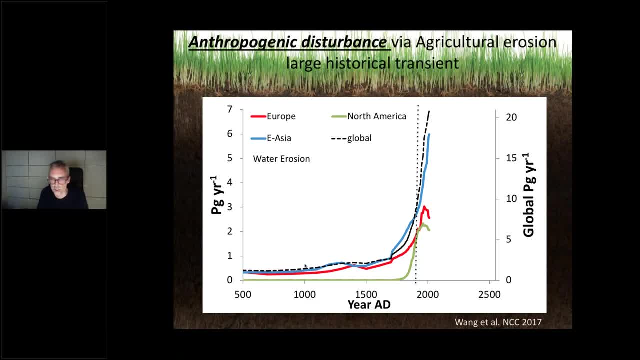 This is, of course, related to the population density, which was relatively low at that time, As you can see, as indicated by the black line here. Okay, So again we have this big increase in soil erosion, in the amount of sediment, and also 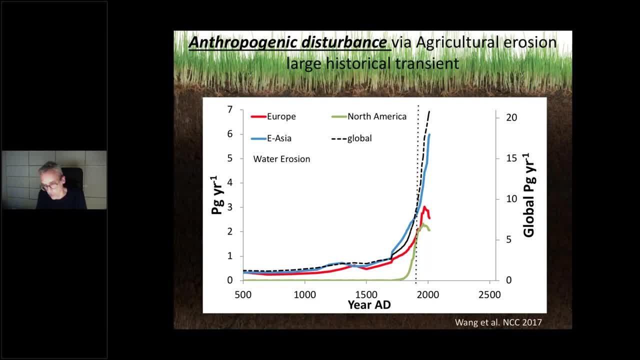 carbon being eroded from our fields, which is again related to the increase in population. And what is interesting to see is that you already see some differences. So if you look at, for example, Europe and North America, we already see the effect of 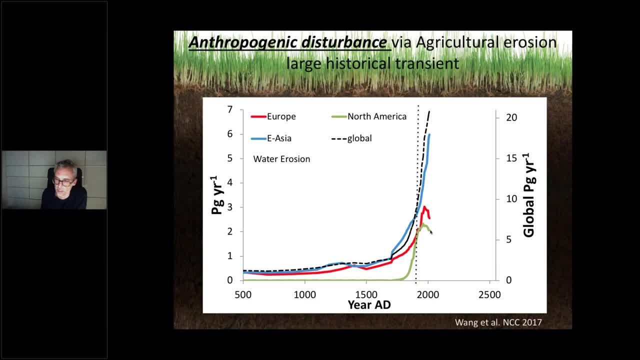 the implementation of soil conservation programs, like in the 1950s, 60s, 70s and onwards. The same can be seen in Europe, But you can also see that for other regions, especially in those tropical regions we are. 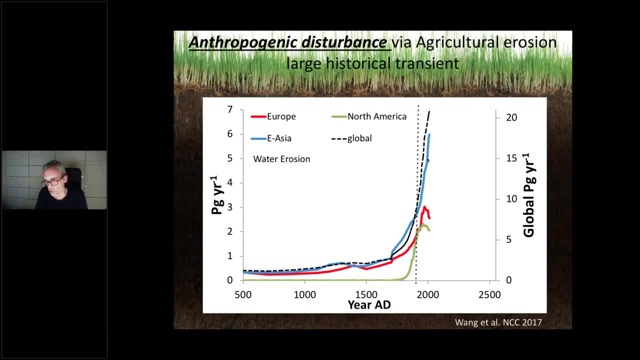 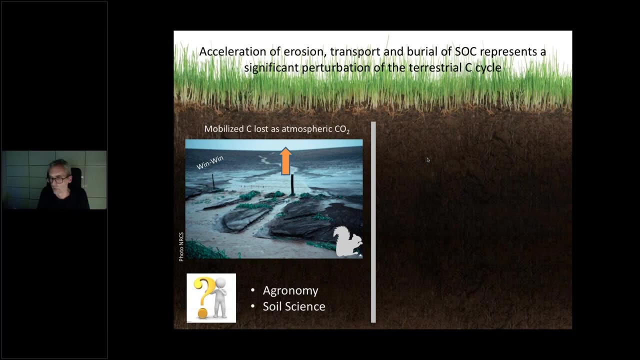 still following the increase of population, So we also expect a quite significant increase in soil erosion rates in the near future as well. Okay, So I framed a bit soil erosion from a global perspective and how important it is, and a bit about rates And where we can expect all of soil erosion. 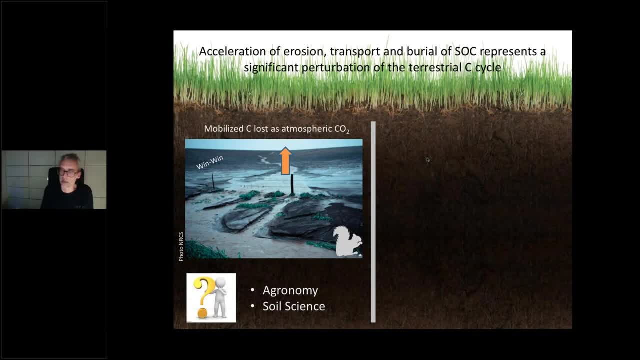 But now I'm going to focus a bit more on how this agriculture, soil erosion- can actually lead to a perturbation of the terrestrial carbon cycle And already indicated in the introduction. there's a bit of a controversy. In essence, there are two schools. 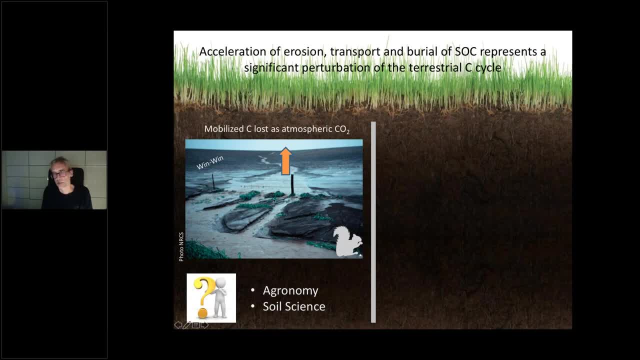 And so the first school basically considers soil erosion to be a significant source of atmospheric CO2. And it is true. Okay, That is because they assume that most of the carbon that is eroded and mobilized- as you can see in the pictures from our fields- that is directly emitted into the atmosphere. 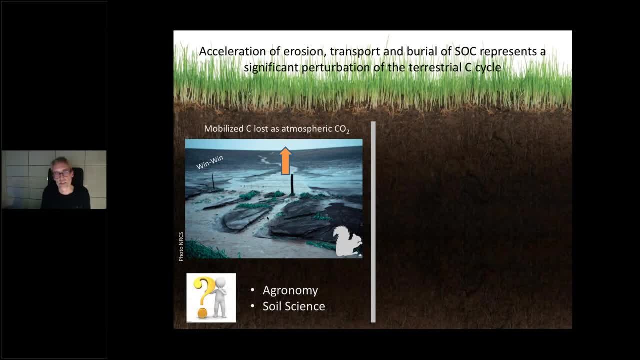 And from that perspective they also consider soil conservation as a win-win, because on one hand, soil conservation can enhance soil quality, soil health and soil functions, while at the same time, if you can stop erosion, you can also reduce. you know perhaps some? 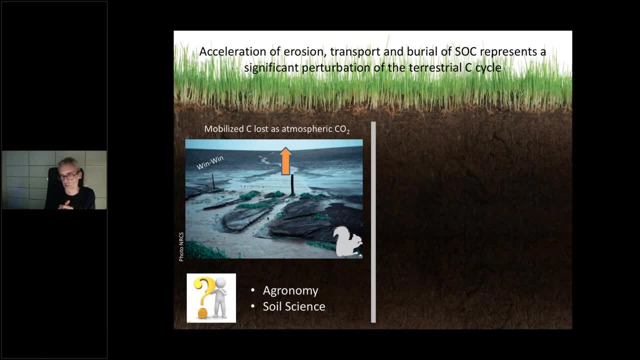 probably small RV damage can also stop or halt this large source, which was associated with the pre-conservation condition, and so that's why they think this is a big win-win. You also see that most of the people that follow this line of thought are from the fields of agronomy and soil science. 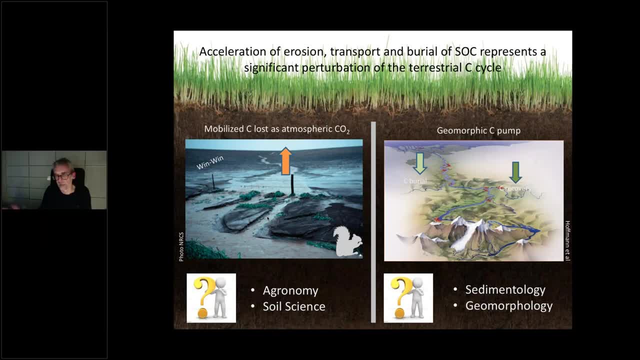 and this contrasts somewhat with other fields and that it's more in direction of sedimentology and geomorphology and what they have actually quite different view. they actually present agricultural erosion not as a source, but that's actually a sink for atmospheric carbon, and they have this concept of the geomorphic carbon pump, which is, in essence, not that. 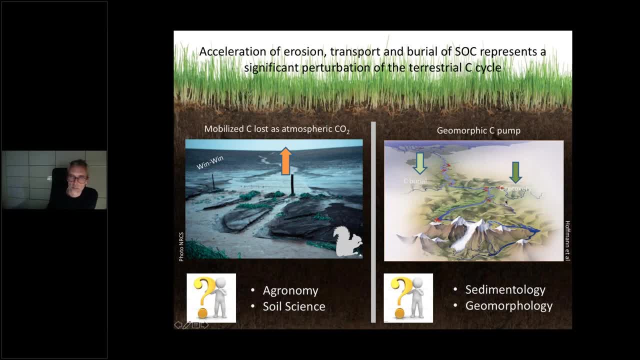 complicated. in essence, they postulate that a substantial amount of the eroded carbon can can be recovered by atmospheric carbon. it can be transported via rivers, to lakes, to oceans, to burial sites, and in those burial sites the carbon can actually be protected from from decomposition, and so the combination of these two actually provides provides a sink. 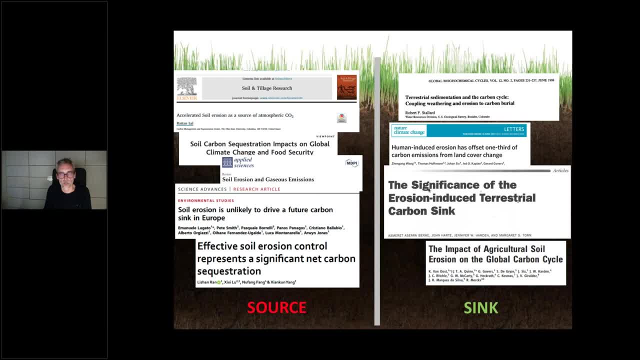 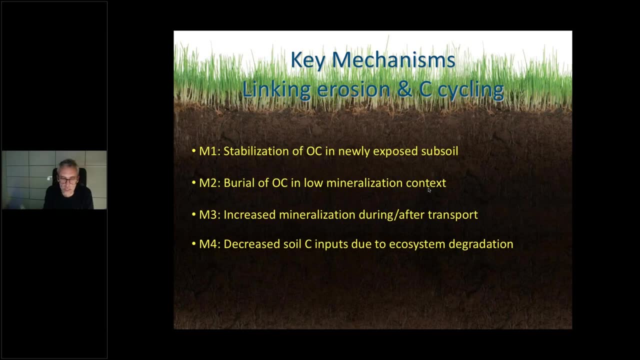 If you go into the literature, you will see that there is quite a bit of controversy, different papers, different approaches, different methods, different models. so it's a bit all over the place, but we're going to go through a bit of the- the process of the research, and the- the mechanisms. 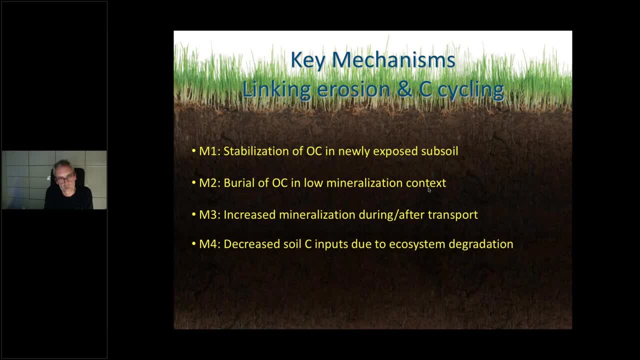 behind the things i'm talking about, and so i would like to briefly introduce to you the mechanisms that actually link erosion to carbon cycling and the four mechanisms which i labeled m1 to m4, and these labels will actually come back in in the in the next slide to structure those mechanisms a bit. 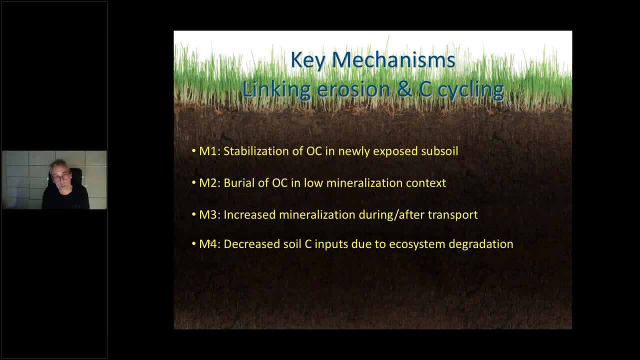 and so the four mechanisms um are behind this link between erosion and carbon cycling. so the first one is the carbon recovery which i just mentioned, so it's a stabilization of organic carbon in newly exposed soil. the second mechanism is also related to the geomorphic carbon pump. 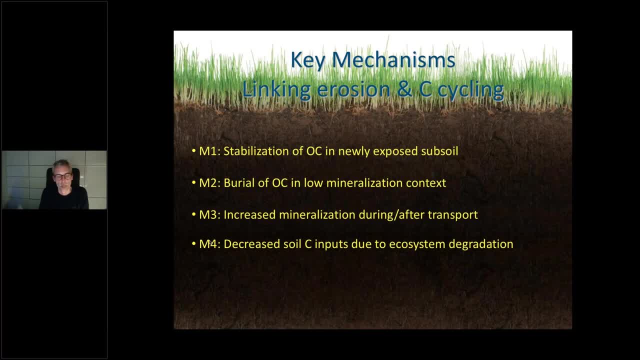 is the burial of carbon in a low mineralization context. the third mechanism is related to the school, which uh postulates that it's a big source. so they suggest that the erosion actually induces a substantial increase in mineralization during and after transport. and also mechanism which plays 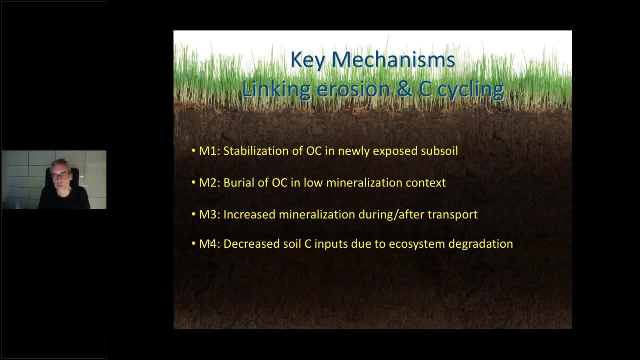 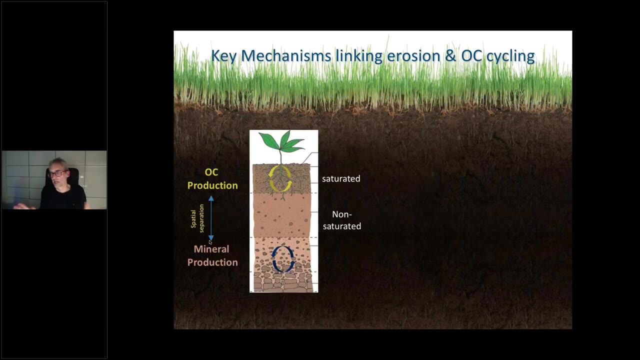 a role is, of course, yeah, with ongoing erosion of your ecosystem, the whole system can degrade to to that extent that plant production is starting to suffer, which will also reduce your soil carbon inputs into the system. um, just to visualize briefly this, these, these are these four concepts in in a 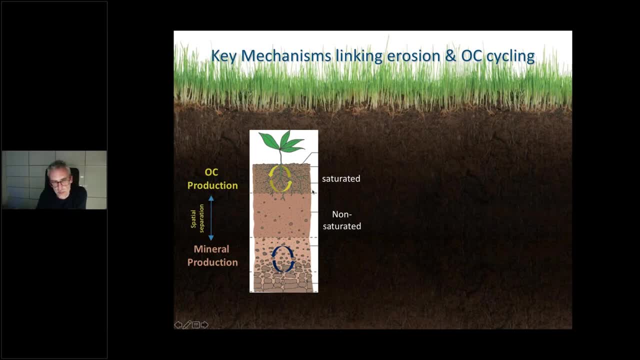 in a sketch um. so what is actually happening? so you have actually a huge amount of fresh organic matter- label material, which is um- in your upper profile layers. it's also one of the biggest flexes in in the global carbon cycle, so about 50 beta grams are respired back into the atmosphere. 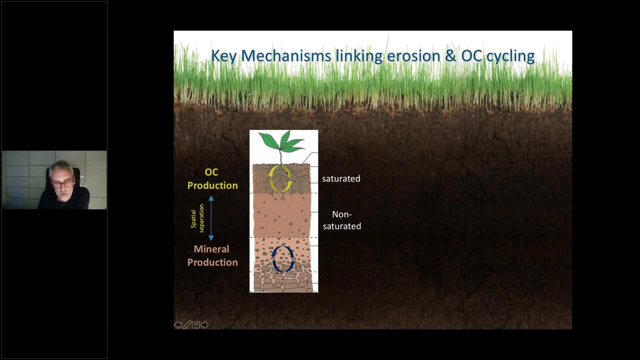 from litter and plant material and they're actually not stabilized to two minerals. um, and why is that? because that layer is to some extent actually already saturated with organic carbon. But if you actually look deeper into the soil profile, this is actually in the bedrock. 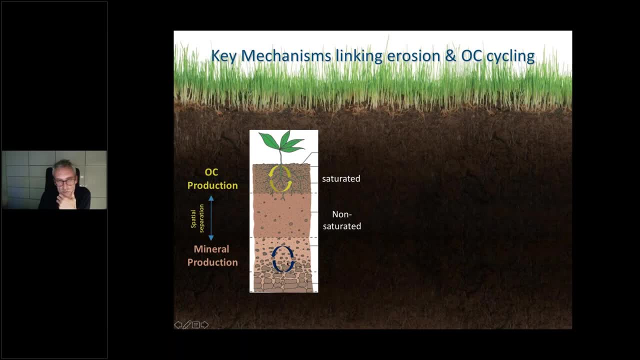 This is where minerals and clay particles are produced. They're not saturated with organic carbon, So in essence, there is a spatial separation between the place where organic matter and carbon is available and the site where actually minerals are available which have the potential to stabilize that carbon. 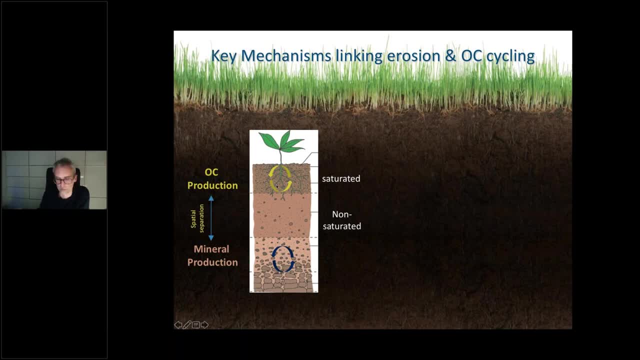 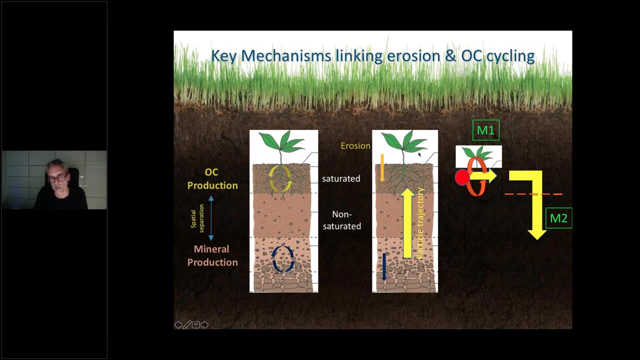 that it's not just emitted back into the atmosphere. So just to visualize this, if we now add the erosion into the mix, you will see that a particle which is subject to erosion would actually follow this from this unsaturated zone where it is not loaded with organic carbon. 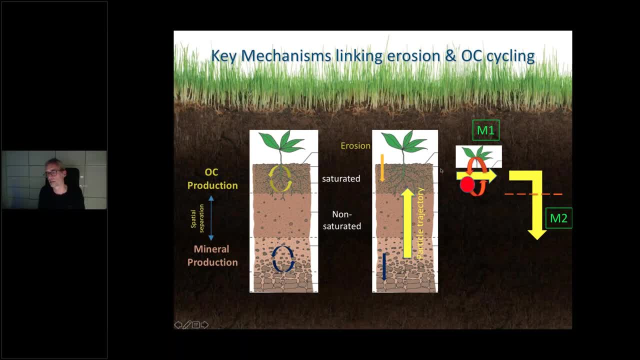 It will be mixed into a zone where this fresh material is indeed available. It will be mixed into a zone where this fresh material is indeed available. It will be transported over the land surface and be buried. So this is mechanism one, this recovery term. 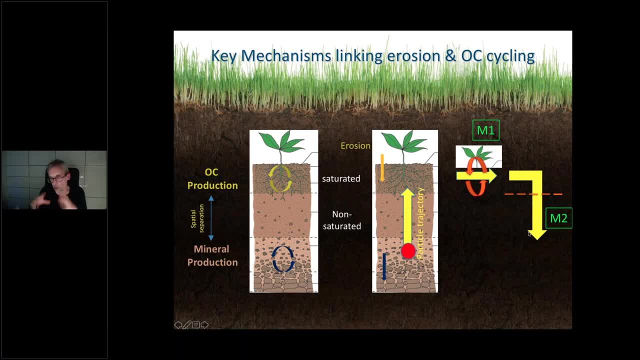 Mechanism two is the burial, where then this eroded particle can be protected from decomposition in a low mineralization, complex, lack of oxygen, high water table. And then the other mechanisms is indeed that during the transport there's quite a bit of carbon being released again into the atmosphere. 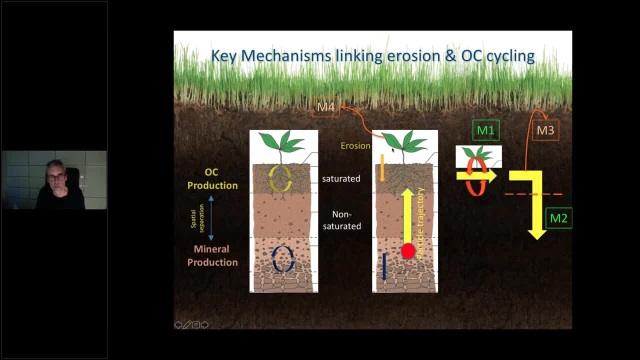 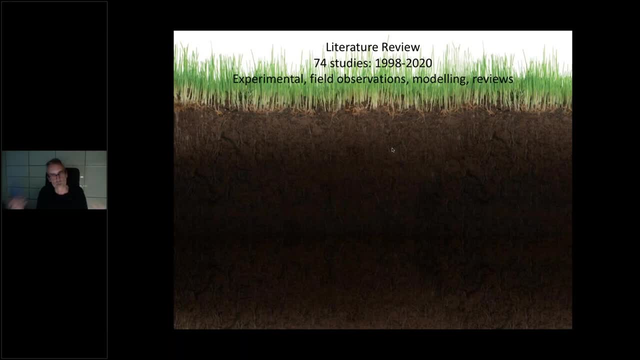 And the last mechanism, of course, is the degradation of your ecosystem. So what I quickly want to do in this last part of my presentation, during a few minutes, just instead of talking about this controversy, we just try to put all the papers that have been published on this topic. 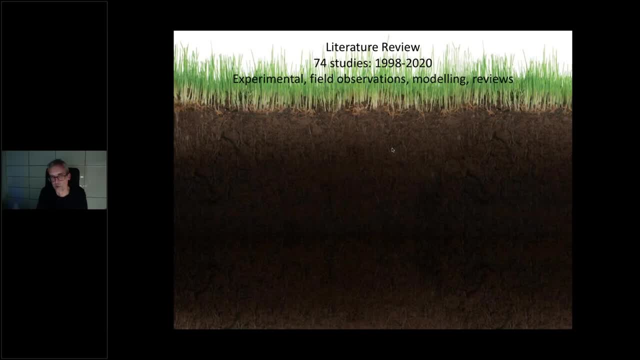 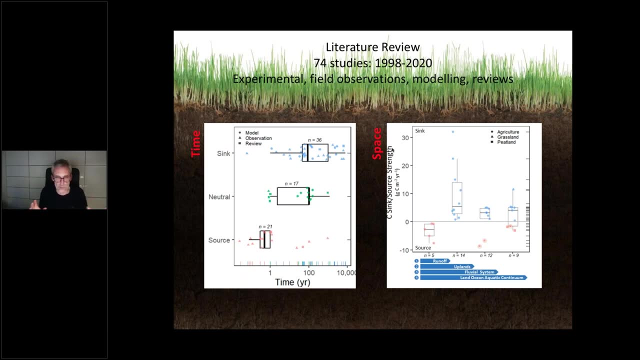 which provide quantitative information into one single framework. And the message I want to give you at the end, in a few minutes, of this presentation, is the following: So this controversy of source versus sink, But actually, if you put all these studies on a time scale or on a spatial scale, 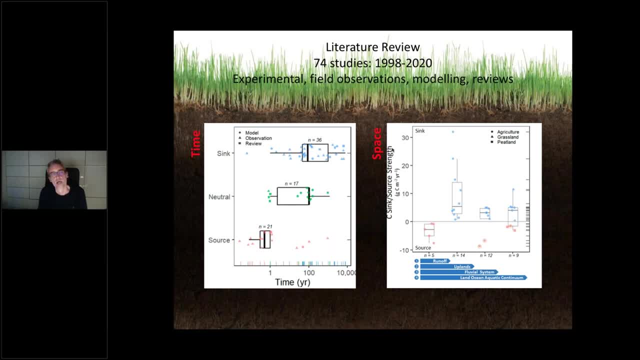 you actually start seeing some structure And in most cases, people who are considering erosion to be a source are usually working on relatively short time scales and also relatively small spatial scales, While the opposite is true- people or researchers or studies that suggest that it's a sink. 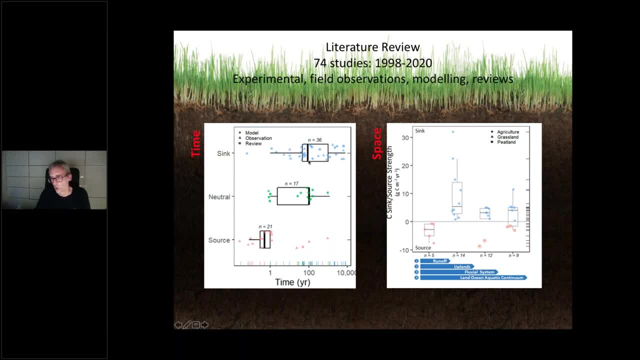 they tend to cover slightly longer time scales- several years to decades as opposed to minutes, days to seconds or years- And they also tend not to just look at what is happening in runoff or on the eroding profiles. They tend to have a bit more of a catchment scale vision on things. 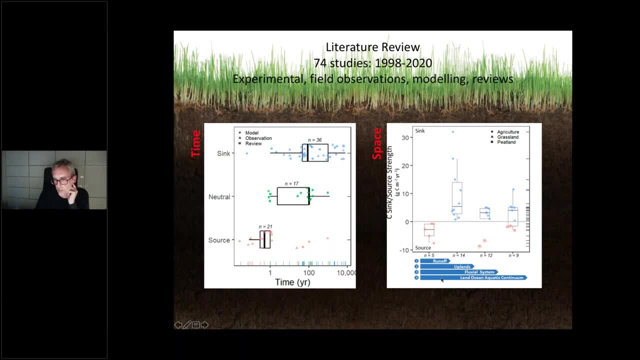 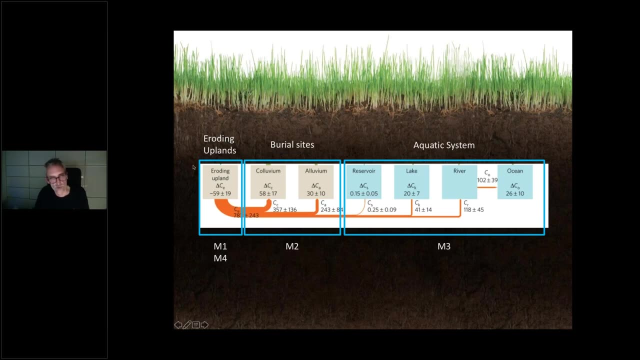 whether they actually integrate the whole system from eroding uplands to the final stage, which is the burial into the ocean. So I will quickly put these four mechanisms on a geomorphic cascade. So we go from the eroding uplands via burial sites to the aquatic system and eventually ocean. 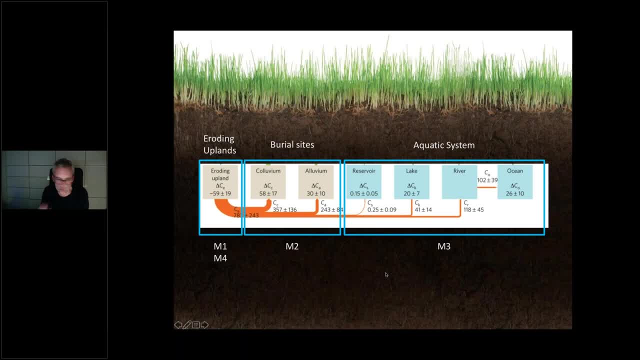 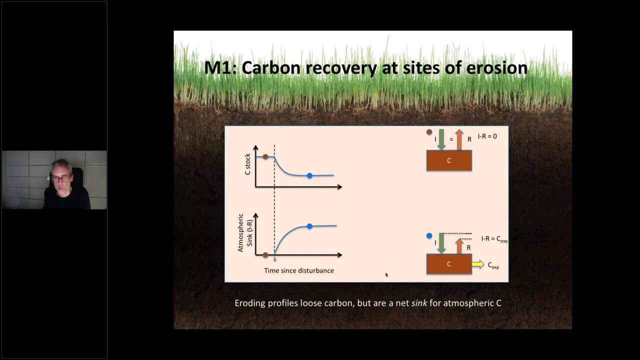 And I will quickly, for those four mechanisms, try to put some numbers on it. So what is, in essence, the carbon recovery at sites of erosion? In essence, if you start from a steady state, a system which is not eroding, 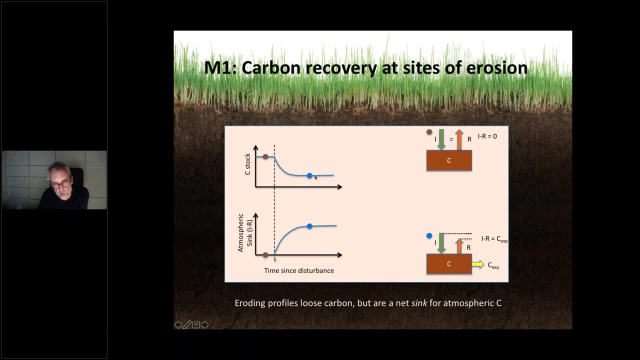 suddenly you start agriculture and you start the eroding. you will see that your carbon stock will go down, But surprisingly, actually, at some point this will reach a new steady state where the erosion or loss is in equilibrium with the input of carbon and the respiration. 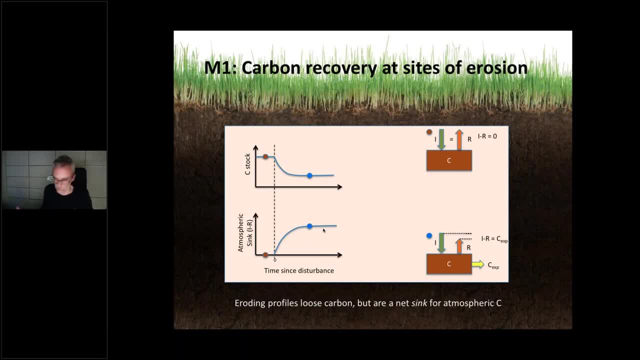 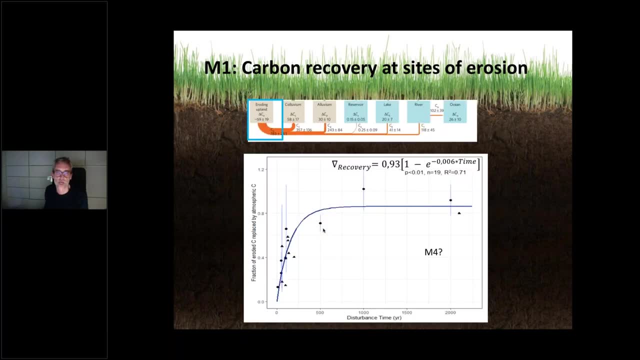 So at that point you actually have a system which is losing carbon. The carbon stock is going down. In essence, it's representing a net sink for atmospheric carbon. And if we look at the data which is at hand in the literature, we can actually see a very similar structure in the data that we have in our concept. 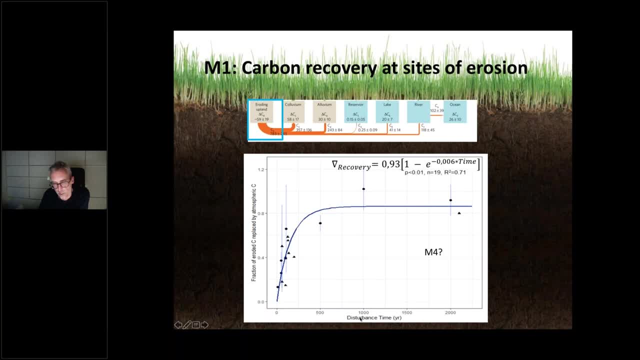 You can see. if you go to systems which have been subjected to agriculture erosion for several centuries, to millennia, you see that the fraction of the eroded carbon that is being replaced is close to one, and these systems are indeed in equilibrium with the erosion disturbance. 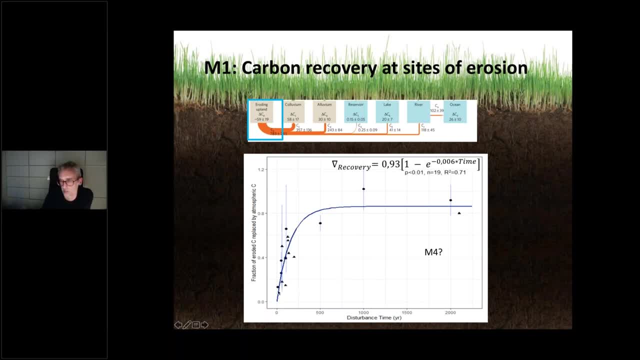 In contrast, if you go to very young systems which are only recently being converted to agriculture, you see that that recovery term is much smaller, and only a small fraction of the eroded carbon is recovered, And so there's also a transient response of an agricultural system to an erosion disturbance. 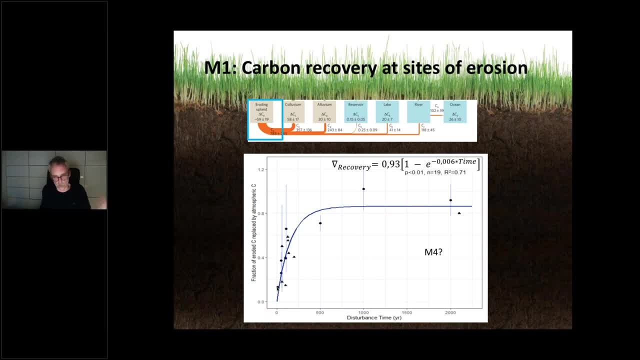 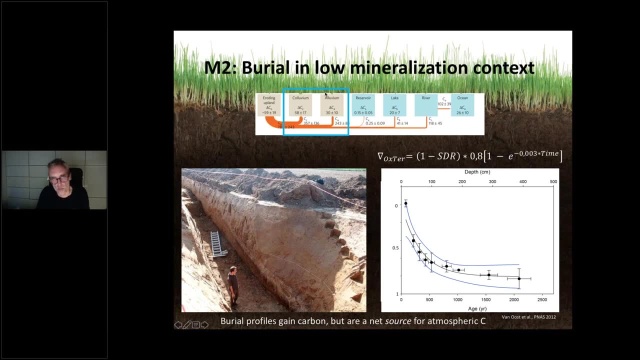 with respect to the exchange of, you know, carbon between soil and the atmosphere. Okay, if you now go to the second mechanism, so we are going down the geomorphic cascade. We went from the eroding uplands and the recovery down to the burial sites. 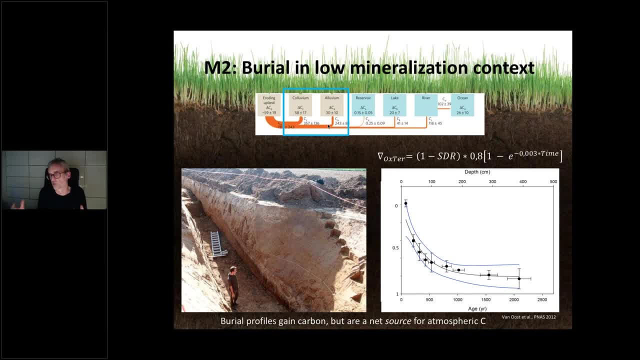 And actually it's also surprising because we generally consider these as sinks for atmospheric carbon, which is true. So the carbon stocks in these burial sites increase because we keep on adding carbon which we erode from the uplands. But actually, if we look in detail at how this carbon is behaving after years, 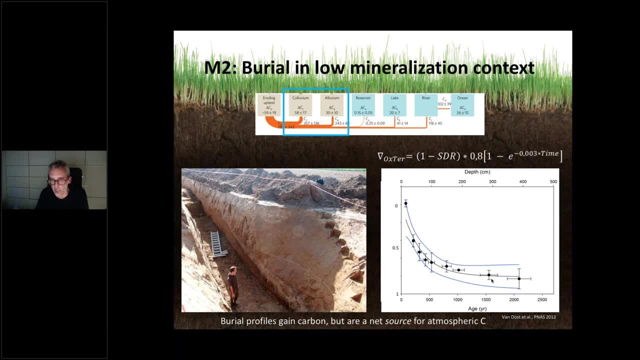 decades, centuries and even millennia. we actually see from the data that actually there's quite a bit of carbon which is being released back into the atmosphere And only a fraction of about 20% is really recalcitrant and can be stored on longer time scales. 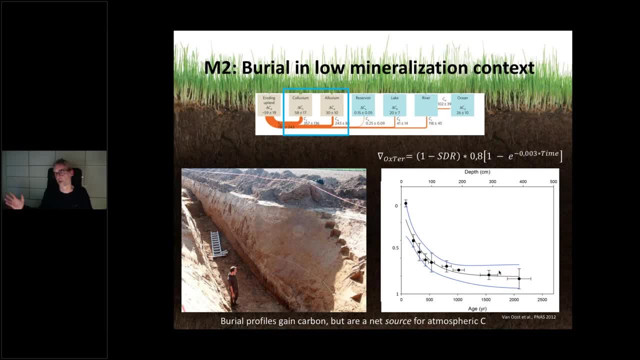 So here you basically have the opposite. So you have a system which has an increase in carbon stock, but the input is lateral, while it's actually respiring carbon into the atmosphere, And so those burial sites, although they have an increase in their carbon stocks, 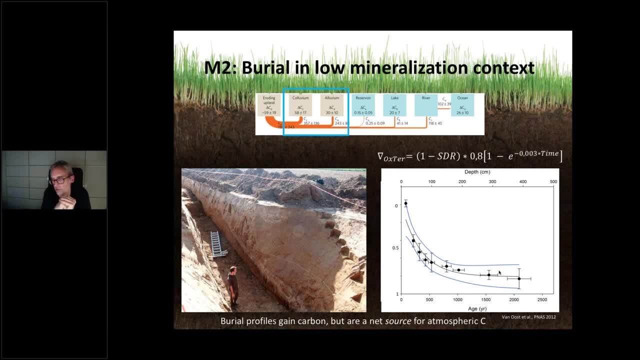 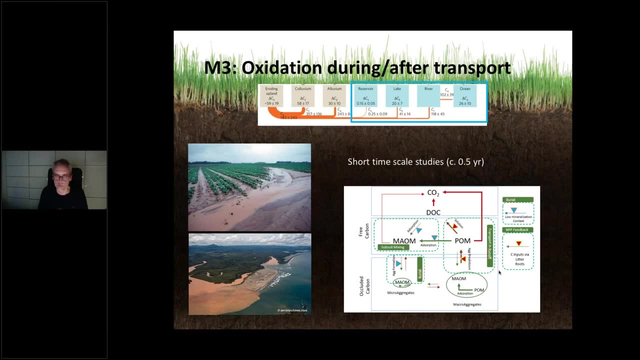 if you isolate them, they basically represent a net source to the atmosphere. Okay, and then the last mechanism, which is unrelated to the school, which suggests that erosion exists, And this is a large source, And so these studies are usually done on very short time scales. 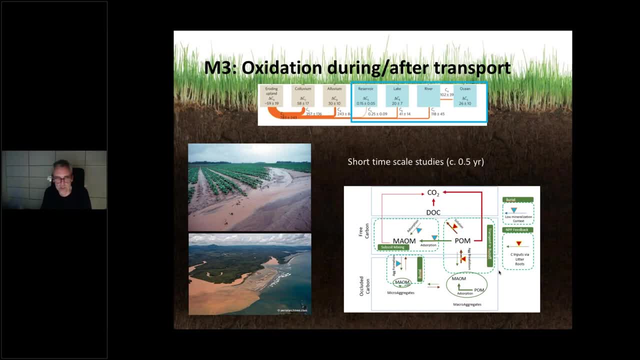 And you can do this in lab conditions or via measurements in runoff, And then you can actually see that this is actually available in the literature, that the loss term associated with runoff and in rivers is relatively small. So in runoff it's only 5 to 10% of the carbon. 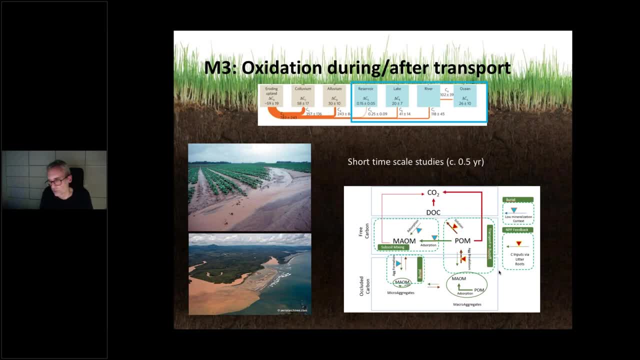 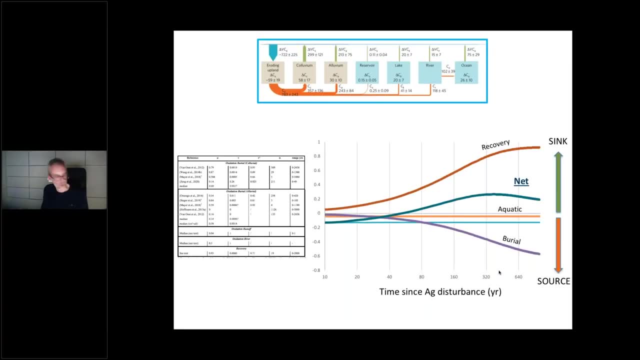 which is being respired, while between 20 to 50% of the carbon that actually ends up in the river is also being lost to the atmosphere. Just to wrap up my story, I see I have two minutes left. So if you put all these different boxes together, 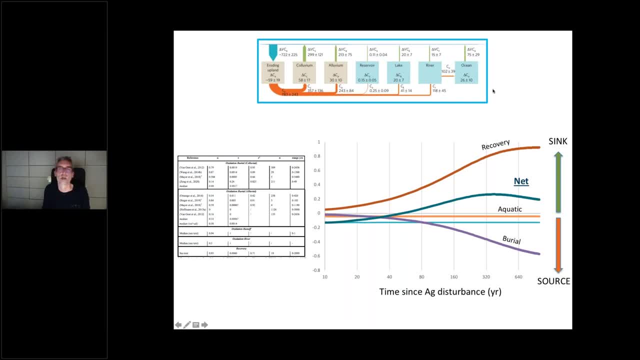 so if we put the geomorphic cascade and all the different responses that I've shown from the different mechanisms on one graph, and so these lines, they're informed by all the studies that we put into our dataset, based on the available data in literature. 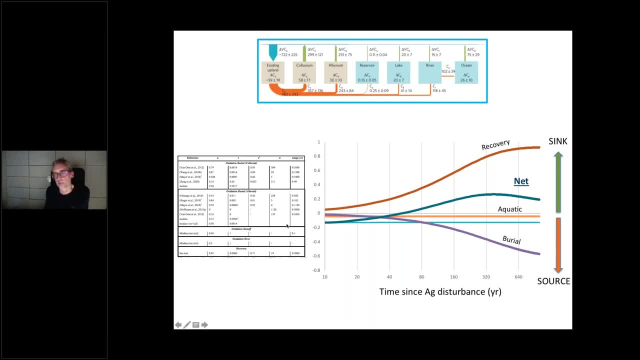 you can basically see two things. So the first thing is that there is also, if we start agriculture here at one and here we go further in time, this is everything representing a sink and the negative is representing a source. The first thing you actually see is: 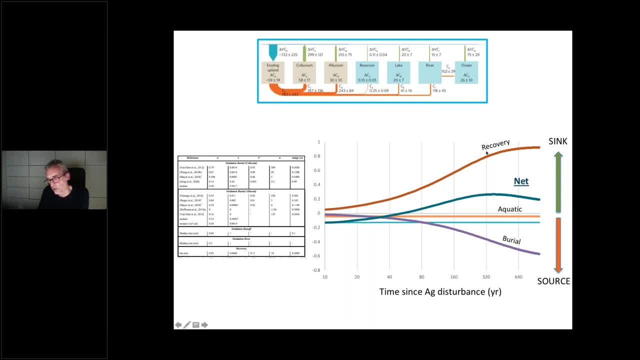 again, you have these transient responses of basically every system, whether it's recovery, the burial site or the net overall effect. if we sum up all the different aspects, The second thing we see is that we have both quite important sources and sinks. 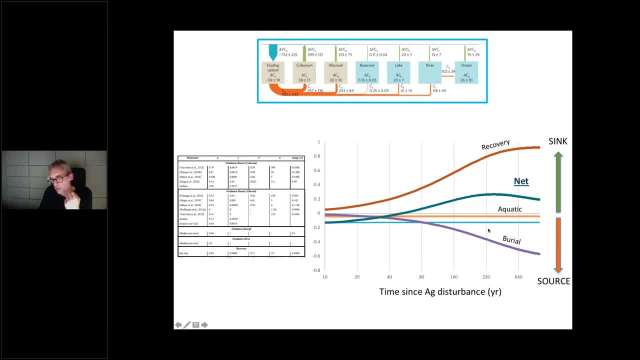 playing at the same time, And this is also why the net effect is actually not a very big source or a very big sink, but it's kind of compensated by both erosion representing a source in the burial sites and during the transport in aquatic system. 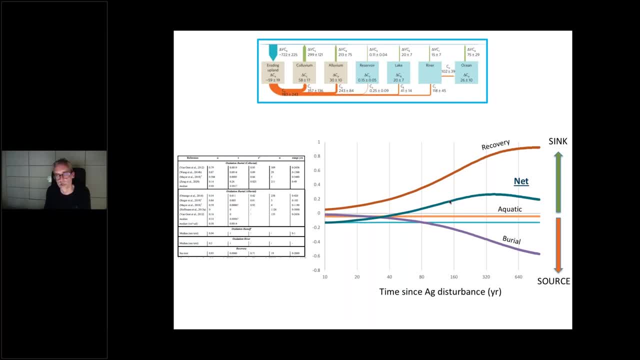 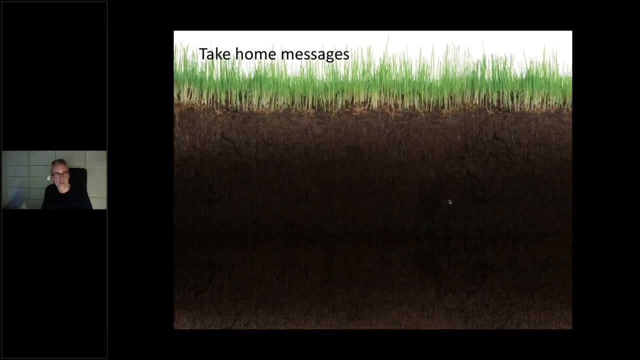 So and representing a sink on the eroding crop lands. So what are the take-home messages that I prepared for this presentation? So I think, to some extent, I think this kind of framework, where we look at different space and times, can somewhat reconcile the apparent paradox. 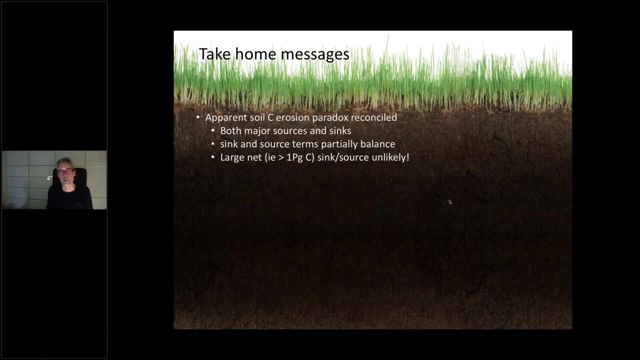 As I just mentioned, we have both major sources and sinks. They are partially balanced, So I think this also means that the schools that represent a huge source or a huge sink associated with erosion is highly unlikely. It's probably a very small sink or a very small source. 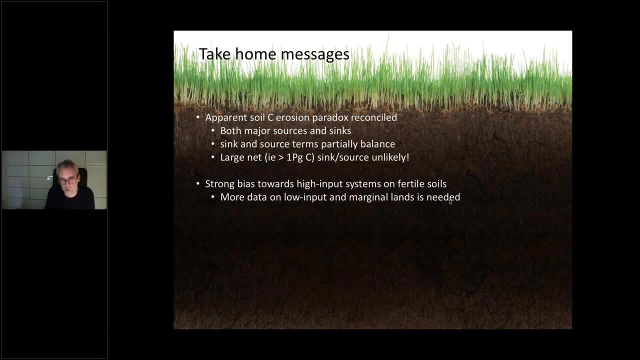 What I do want to mention here is that most of the data that we found in the literature actually comes from high input systems on fertile soils. So there's much more data that we need to have on how systems in low input, how systems respond in a low input soil. 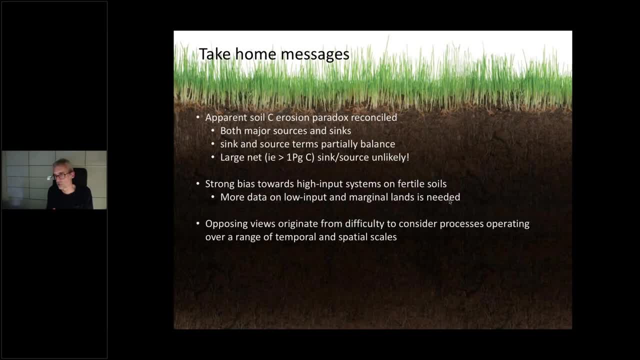 So I think this is a very important point that we need to think about in context. So, as I already mentioned, so I think the opposing views and the controversy basically originates because we're having processes that operate at different space and timescales. 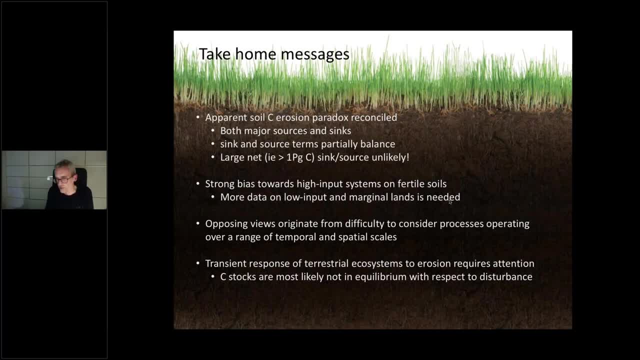 So that's not very easy to synthesize. I also put emphasis on the transient response. So a system which is subjected to erosion is most likely not in equilibrium, which has implications for current sequestration studies. So I would like to end my presentation. 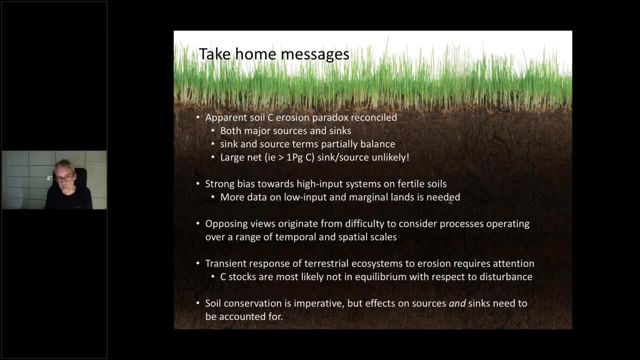 I see, on time with the message that, of course, soil conservation is imperative. We need to preserve our soils, we need to enhance our soil functions, but we cannot just ignore both the sources and sinks which are associated with carbon erosion, And so it's not a big win-win. 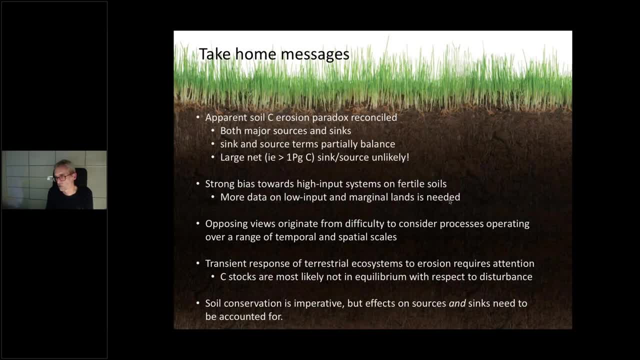 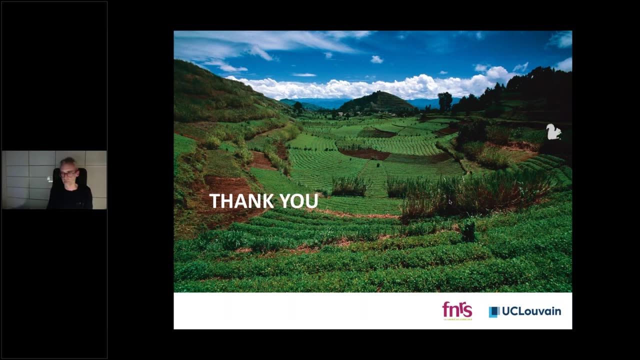 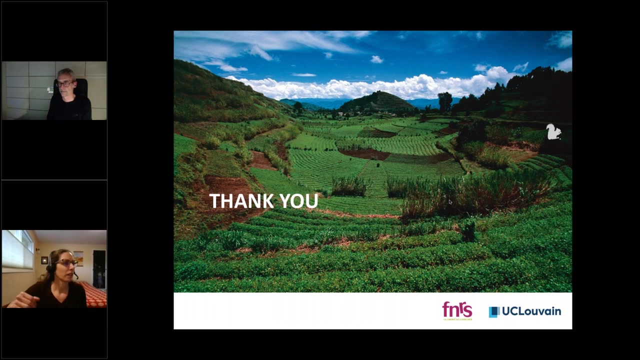 It's not a big sink, neither It's probably a small sink or a small source, And this needs to be considered when we talk about the effect of erosion on carbon sequestration. All right, I thank you for your attention And I'm happy to take any questions you have. 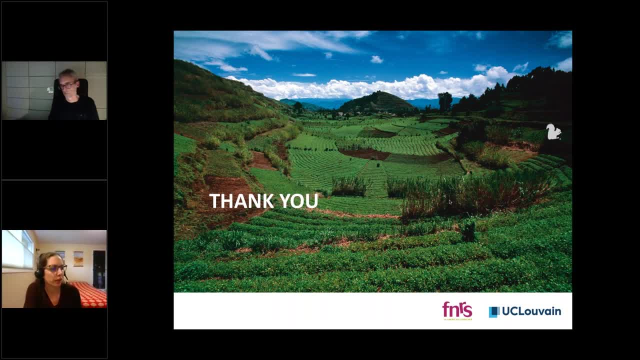 Thank you so much, Christoph, And all the folks that are attendees. I would invite you to post questions into the questions section And I'll put the link to the question section of the GoToWebinar control panel And I can pull some questions from there. 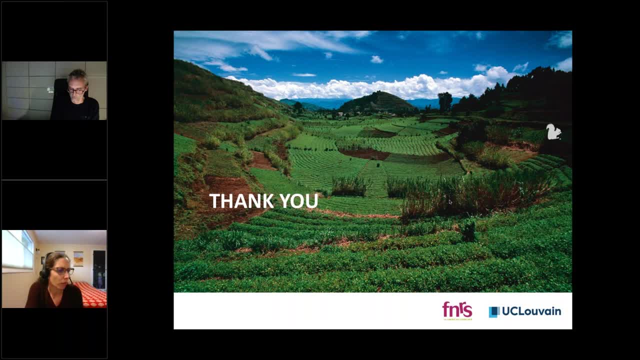 Looks like we do have a couple. There is one question for clarification question: Could you describe recovery? Is this recovery of a plant community, or recovery of a new equilibrium, or some combination of that? No, When I use the term recovery, it basically refers to the recovery. 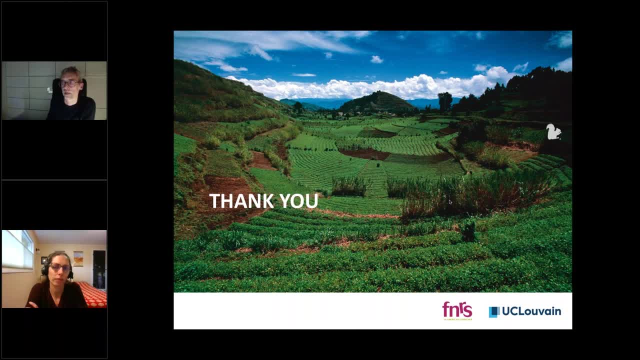 of the organic carbon content in the soil profile And so soils which are being subjected to erosion they lose a part of their soil organic carbon, But via continuous plant inputs a part or the total aspect of that lost carbon via erosion will be replenished. 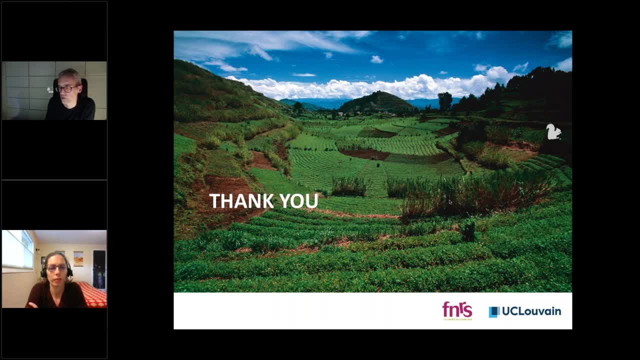 And so, in that sense, soils can recover from the erosional loss, And that's the meaning of the word recovery for me. Okay, great, And then a question from me. So I think many of our attendees have maybe a preoccupation focus. 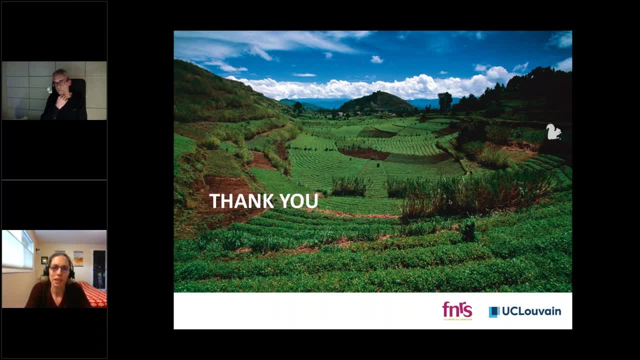 on what's happening with emerging carbon markets and the quantification of carbon change, Which I could say serves two purposes, right. One purpose is to incentivize certain practices that we want to see more of because of their multitude of benefits. But then the other purpose of it. 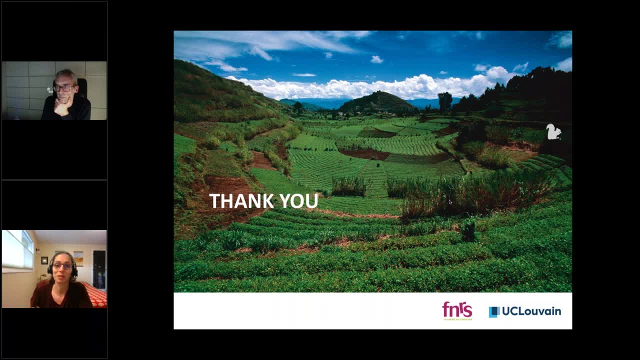 is to actually provide robust accounting to help stem emissions overall, And what is the role of accounting for erosion? And that's a really big question, I know. So I guess I would start with, you know, with the time horizon of carbon credits being five to 10 years, 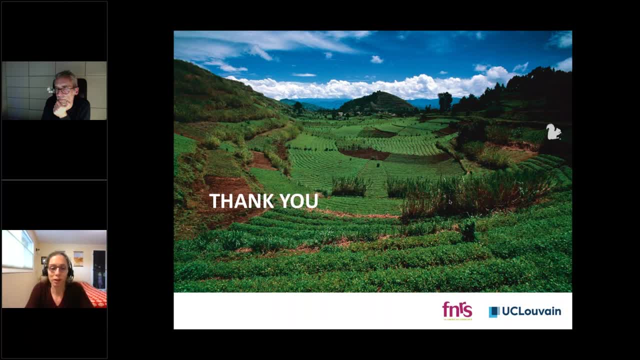 do you think that there should be accounting for carbon changes that are due to erosion? But, to be honest, no, I don't think so Because, first of all, I don't think it's representing a major effect, whether it's a sink or a source. 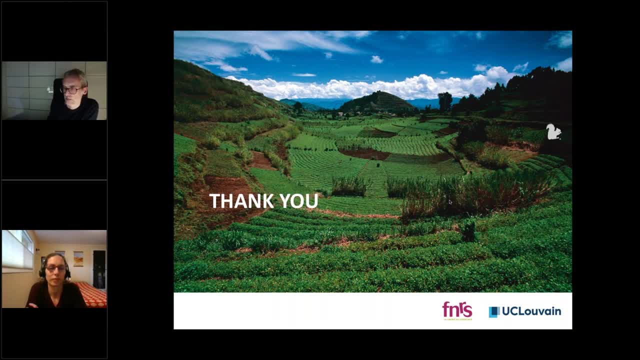 It will be a very small one which is very difficult to detect and to prove and to monitor. So from my perspective I don't think it makes sense to include that in those schemes. But I do think if you really want to measure and monitor soil carbon sequestration. 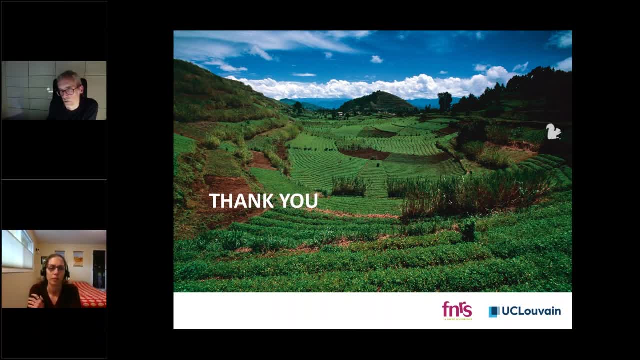 and you need quantitative proof to what extent your ecosystem can capture carbon into soils. if you work in eroding systems, then the measurements will also be largely influenced by the amount of erosion and the lateral loss of carbon soil carbon via erosion, And that's something which needs to be considered. 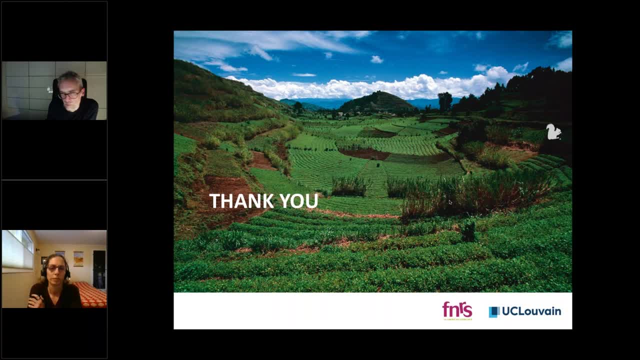 Otherwise, your monitoring scheme will be biased, And it's not only representing the vertical fluxes and the direct exchange between soil system and the atmosphere, but you also need to consider that there is also lateral movement, And so that's an implication, I think. 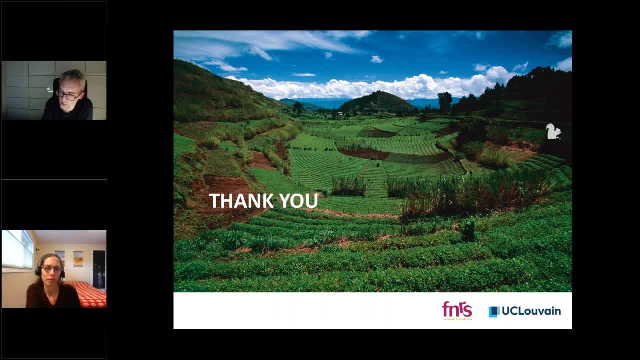 which is directly relevant for carbon credits and soil carbon monitoring programs. Okay, great. And then, Oh, there's some good questions coming up here, I'm going to jump in. So Jen Harnon asks: in your Mechanisms 1, through Mechanism 4,: 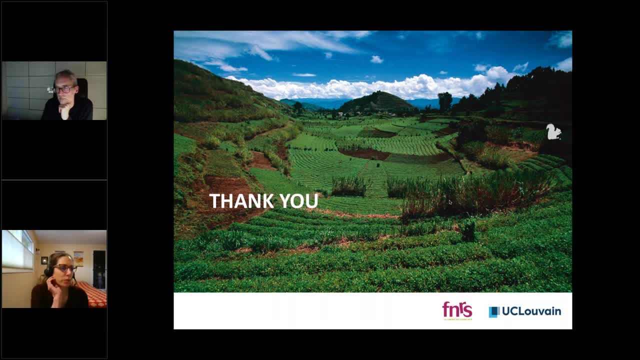 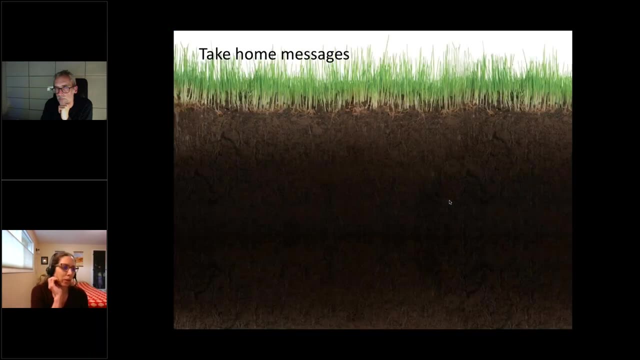 you generalize that inputs to soil are likely reduced as a result of erosion. She says actually in fertilized lands and phosphorus and potassium-rich subsoils. this seems overgeneralized. Are there also studies that account for increases in inputs during erosion? 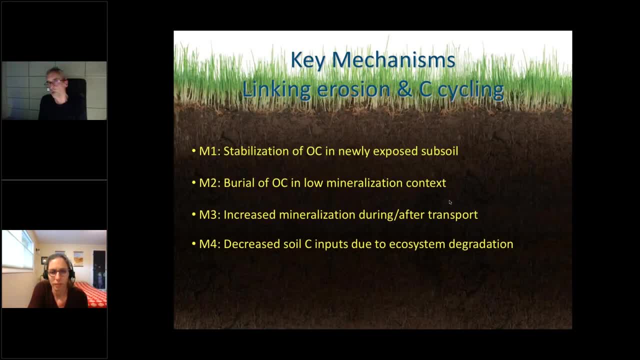 So I'm trying to find, I'm trying to understand the question: Are there systems where there is an increase in inputs due to erosion? I think that the general direction of thought is that erosion has a negative impact on soil health, So I find it harder to see that. 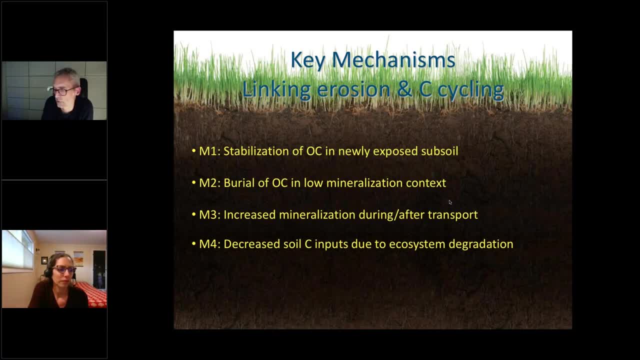 that could actually lead to more fertile soil. unless you're kind of eroding in a very specific condition where we have like a Bt horizon which is clay enriched, This is possible. but I think these are more exceptions than general rules And the only thing I maybe can add to this: 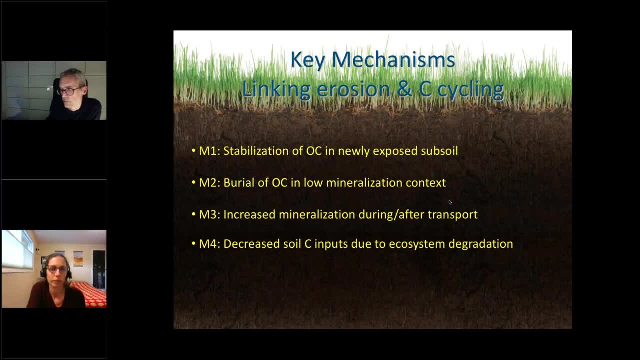 so I think the data that we have is indeed from high input systems, where those negative effects of erosion are completely masked by the fertilizer inputs we provide in our soils, And that's why it's also probably highly like- more likely- that in low input systems. 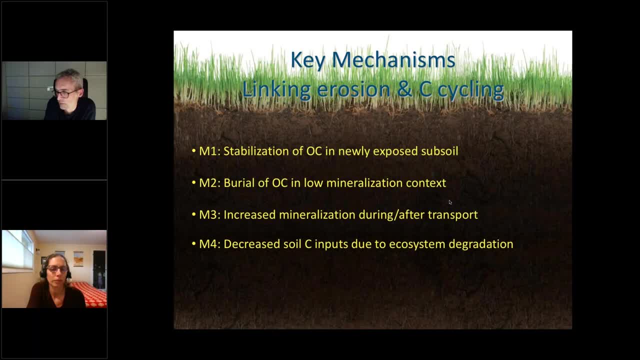 that recovery term will not be as big as we have in high input systems. So that would be is probably much more important, But in a negative way, I think, not a positive. Okay, great, Yeah. So here's a question asking. 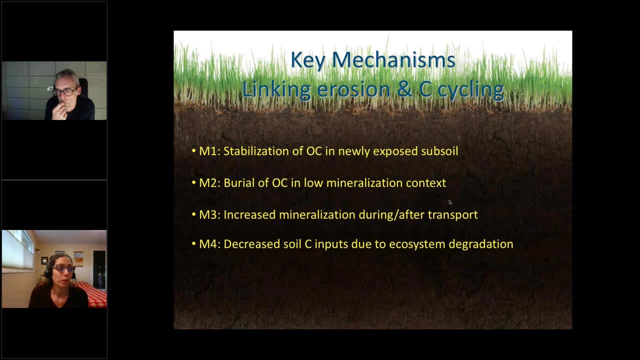 about the impacts of urbanization on erosion rates In your group's work. have you identified any differences in urbanized versus non-urbanized areas in terms of erosion rates and carbon impacts? That's a difficult one. We I have not done any research in that aspect. 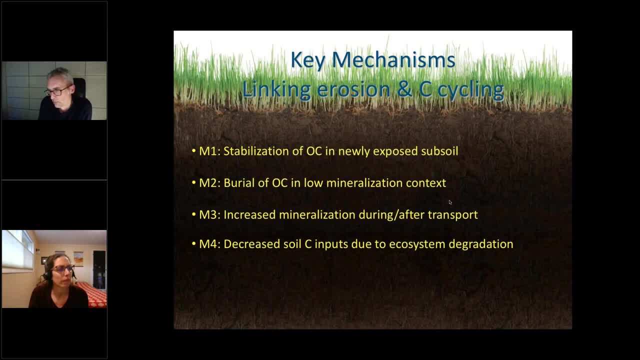 I know it's an issue, But I think, surface-wise, the area being cultivated in croplands and subject to erosion is orders of magnitude higher than the surface we have in cities. So I think that's the reason why I think most of these studies. 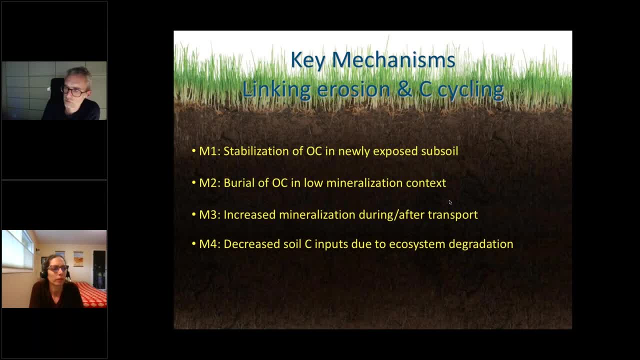 they focus on agricultural systems and not urbanized systems. But I have to be honest, I cannot provide a decent answer on that question. Okay, great, That's an interesting one. Yeah, And there's several questions that are kind of trying to get a handle. 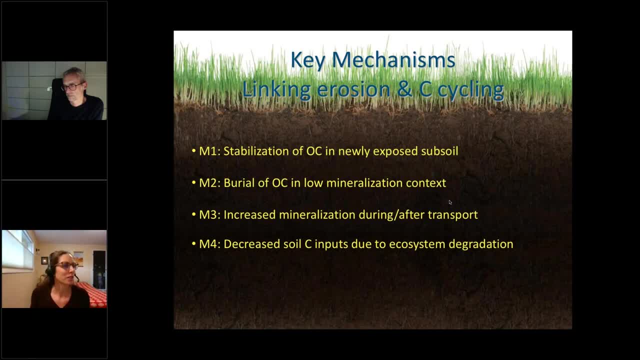 of orders of magnitude of different situations. So one question is: does wind erosion or water erosion contribute more to to carbon movement and sink and source dynamics? Yeah, On a global scale, by far water erosion is the most important process. Yeah, 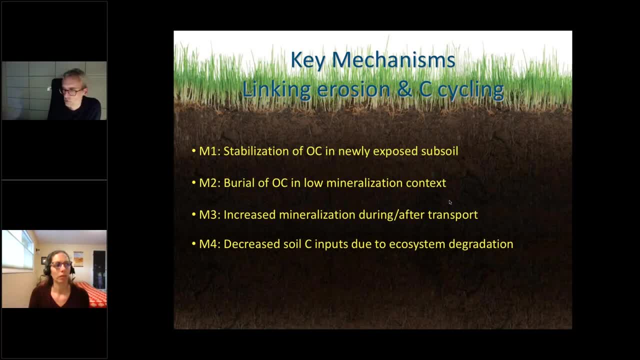 I don't have the numbers here, but it's, I think, close to one order of magnitude more important, But it's in very specific conditions, like in the Midwest or in Australia or in Africa. Of course you do have regions where wind erosion. 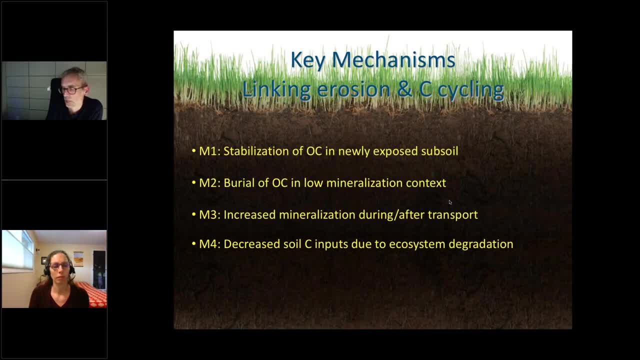 is indeed more important than water erosion, But on a global scale, water erosion is by far the main agent to mobilize and transport soil and organic carbon, But of course you have regions where that's not the case. That was really helpful. 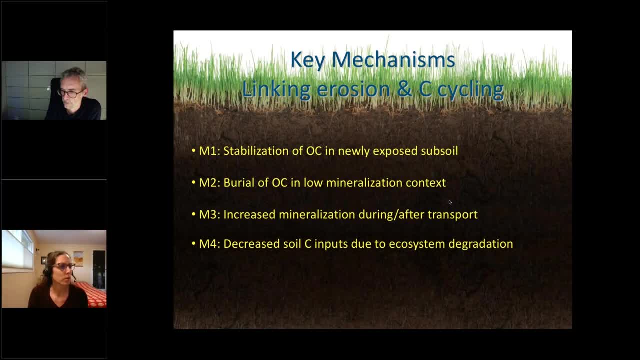 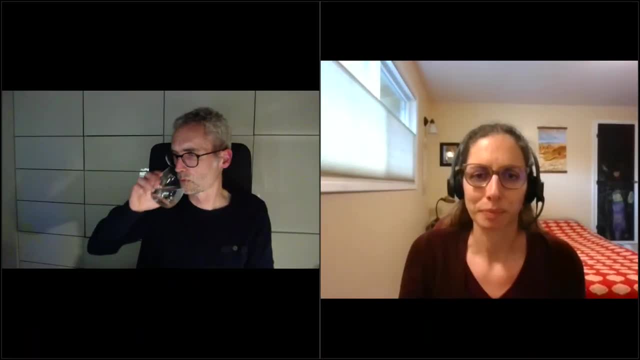 Thank you so much, Christoph. I'm going to go ahead and pass presenter mode to Ken now, And there'll be a little bit more time for questions too at the end. So, Kenwin, you have a chance. Turn your webcam on. 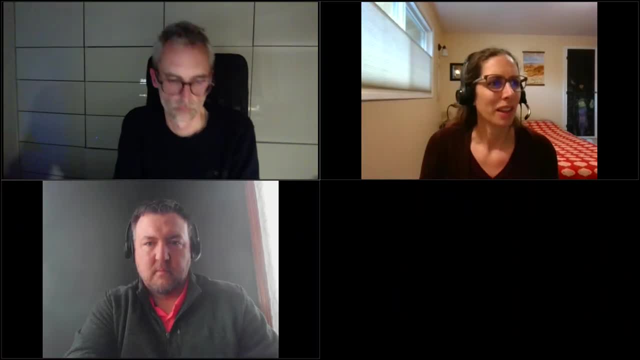 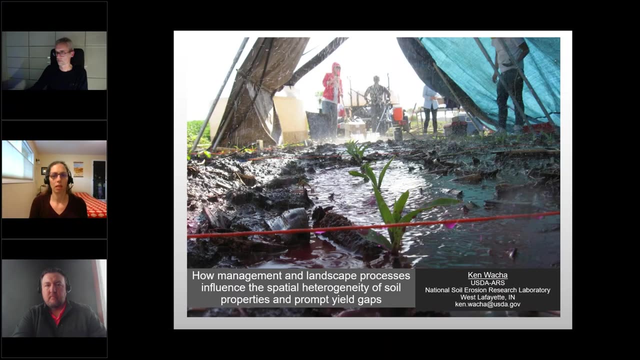 And then I, there you go. And then did you see the invitation to take control. Yep, Okay, Is that showing up? Yeah, it looks good, Sweet, Okay. So, Kenwin, you have a chance to turn your webcam on. 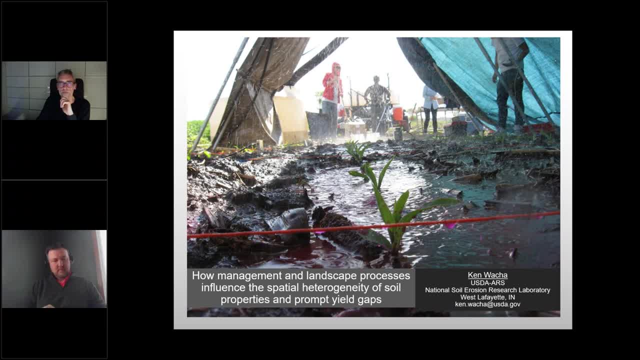 And then there you go. And then did you see the invitation to take control. Yep, Okay, Is that showing up? Yeah, it looks good, All right, So let's get to our 20 minutes, All right? 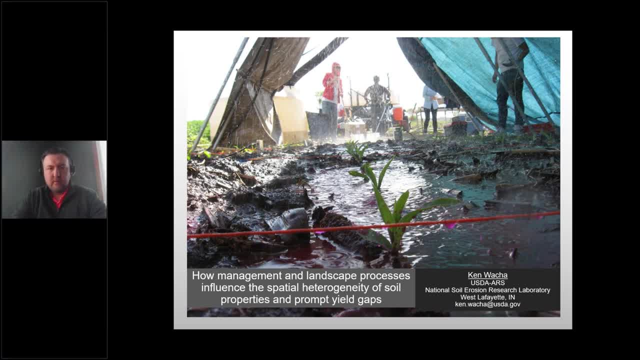 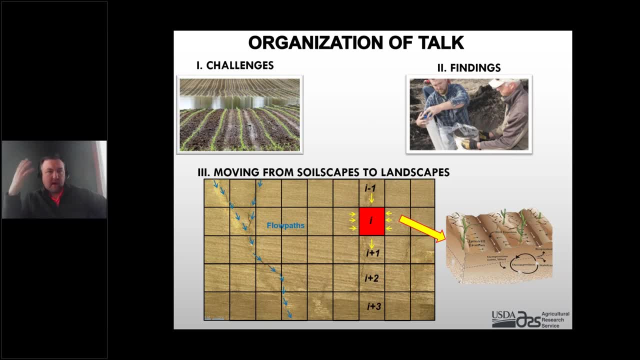 So I'm going to give a little talk about kind of my, my thinking or how I let this stuff roll around in my head about erosion, the process of erosion and how it kind of shapes a lot of our landscapes or kind of our distribution. 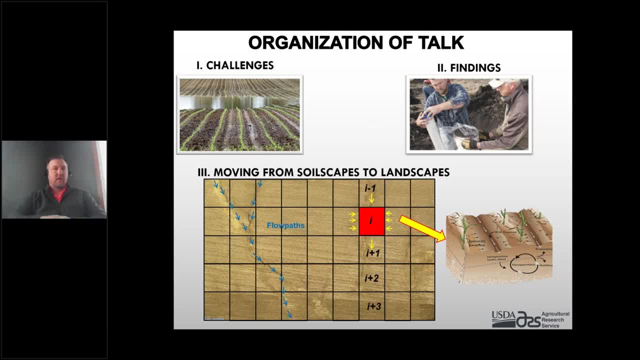 of properties, you know, production and so forth and so forth. So, Kenwin, I'm going to start off by talking about some of the different landscapes I've seen in the North and South and all across different landscapes and kind of some thoughts. 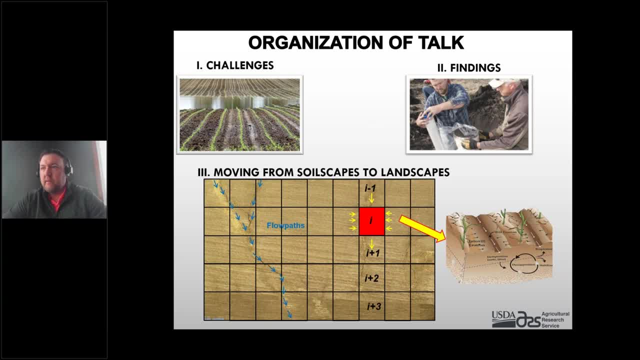 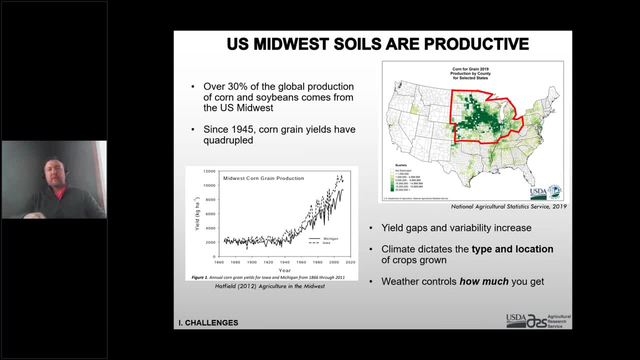 I have, as I've been, you know, doing some field research and rainfall, and so I'm going to focus in also on the Midwest. So, US Midwest, we produce a lot of corn and soybeans. You know it's a global. 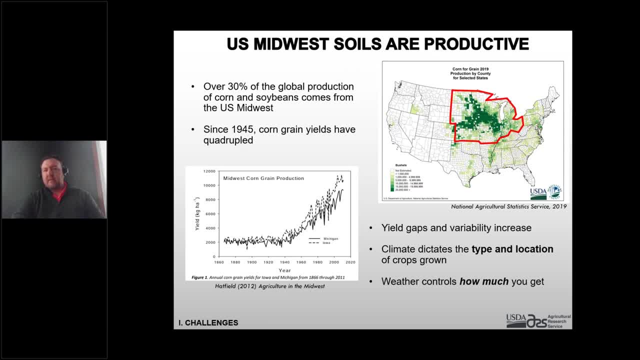 reporter, you know significant amount You see on that image. there to the right it's outlined in red. that's kind of our Midwest there and the takeaway there is: the darker the green means the more corn is being, you know, produced there. 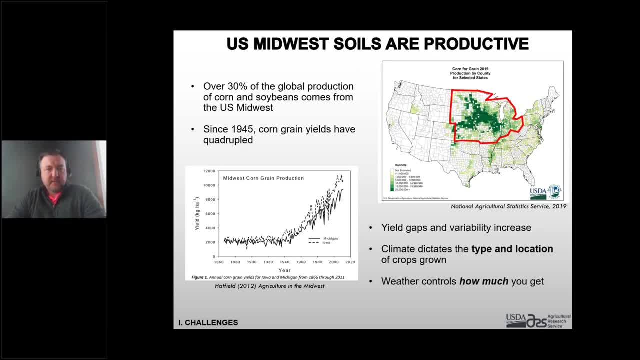 So we see kind of the traditional or the history of our grain production there You see a sharp ramp coming up around the 1950s. So things dramatically shifted there from our normal production to much higher, and which much with the much higher. 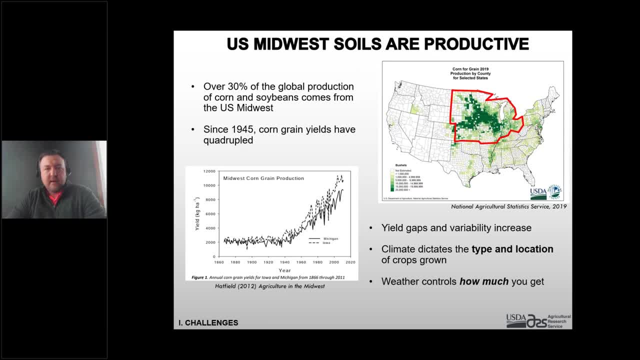 becomes a lot more variability and a lot of that is driven by intensification and kind of its response that we're going to have from climate and weather. So climate, I think if you could think of it as across your you know, like if you're. 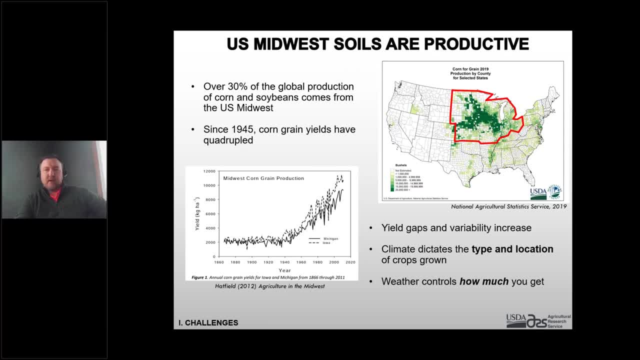 looking at that map up there, it's going to tell you where you're going to grow your crops and what type of crops- or weather- which you don't really have you know that much control over- is going to kind of tell you how much you're going. 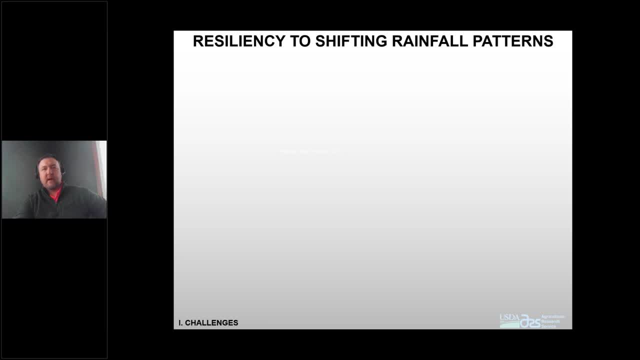 to get out of that crop that year. So resiliency to shifting rainfall patterns and rainfall patterns and how that applies to water-driven systems and how that impacts your climate. So now I'm going to talk a little bit about the changes. 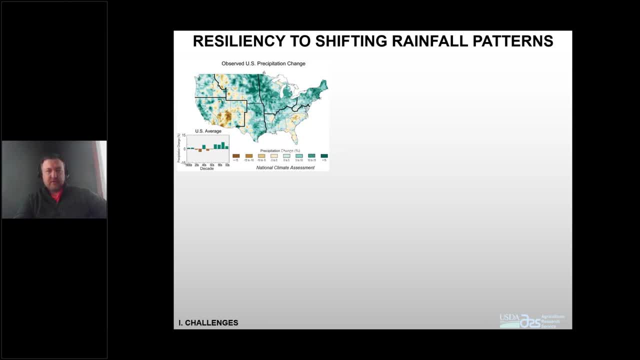 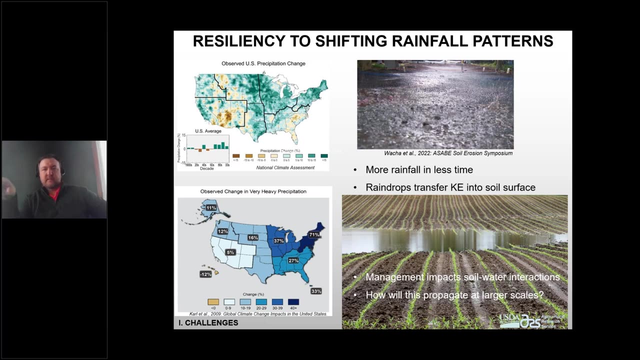 that we've made over the last 20 years. So the changes that we've made over the last 20 years are from observed precipitation change. Darker the green means more is coming. You're going to get more rain, but it's going to. 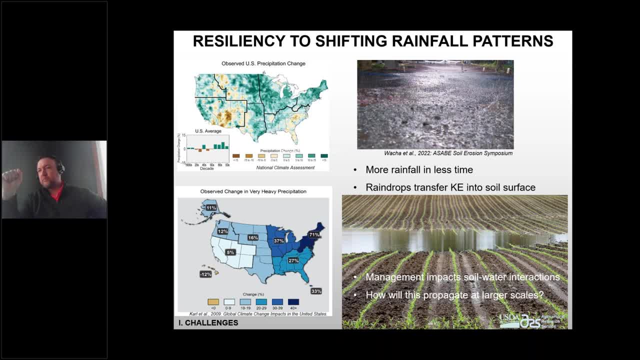 come in a shorter amount of time, And when that comes, you got your energy from these raindrops, So the kinetic energy from falling drops is going to just smash into your soil surface, and that's the instigator of all the erosion processes. 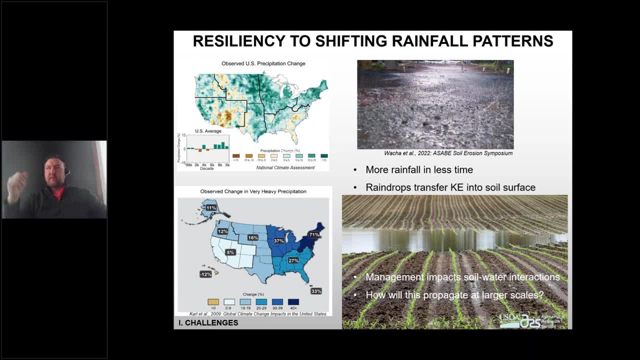 right. So, based on your rainfall intensity, drop size and you know when it happens within the year, you may have windows, where it's very important, with residue and left on the fields or crop canopies or, say, a cover crop. 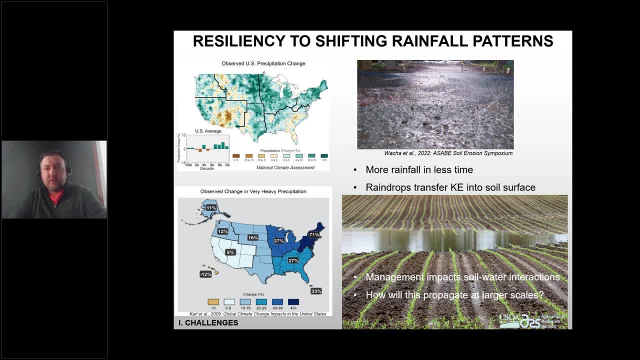 canopies, something to shield that energy when it comes down and you know you stop it right from its first instigation of the erosion processes. So in the bottom right picture there kind of a. this is a common site around much of our area. 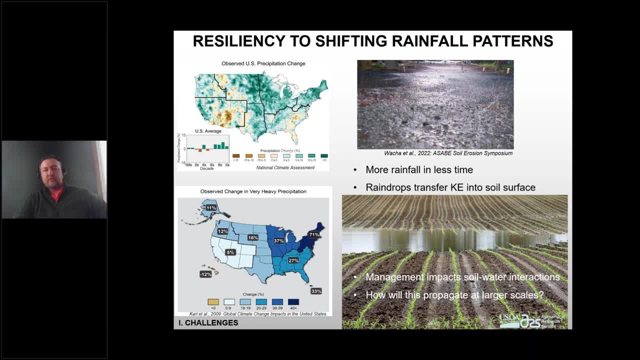 around here after big rains, You'll see, if you look at those initial drops and just hammering that surface and causing some sealing effects, and then to think about, not just within a field but if you look at a whole system, how will some of these interactions 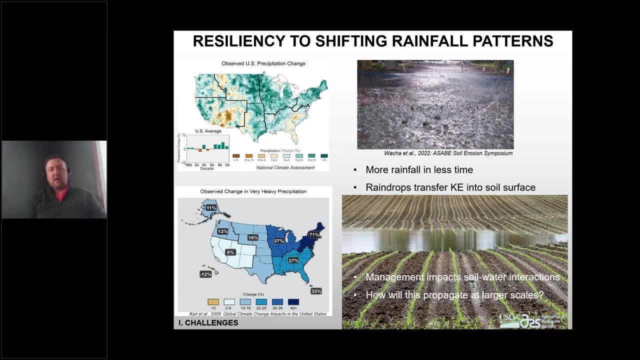 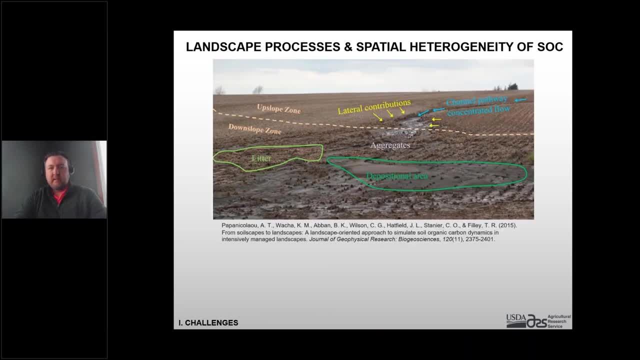 of the of the changing precipitations, the high intensity rainfall. how is that going to propagate as you go up in scale? So I like this picture up here. It kind of shows some of the problems dealing with high spatial heterogeneity. 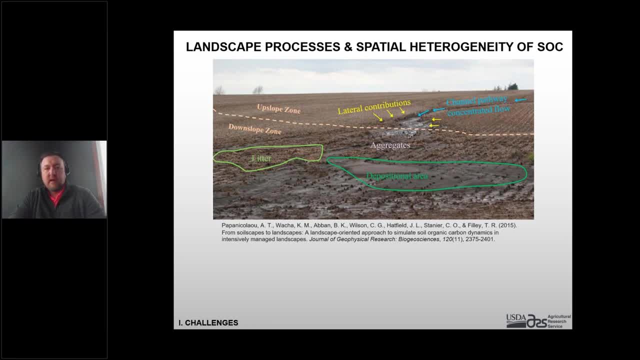 So, basically, if you're going to take soil samples within a field, and you're going to have one sample is probably not going to give you an idea of how active your, your landscape, is. So there's lots of little things drawn on there. 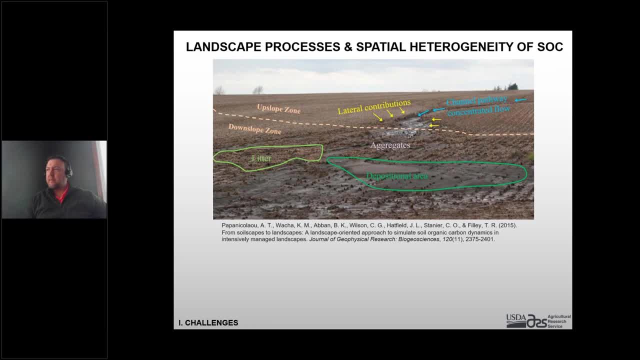 but what I want to show is that you know your topography kind of shapes, how your water kind of runs, in different different controls that could stop and regulate water. That's going to kind of shift and kind of help to delay some of those. 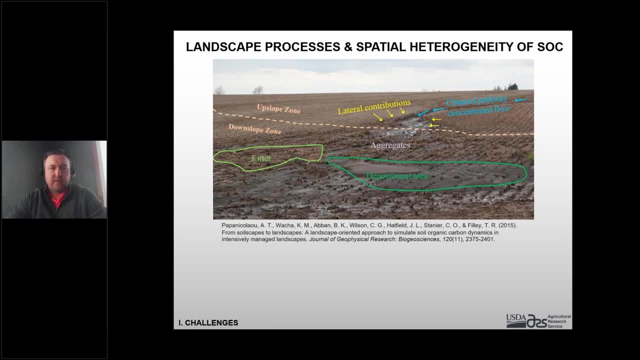 processes and allow more water to go within the soil where it belongs. So you'll have concentrated pathways forming, you'll have lateral contributions, you'll have splash erosion, you'll have the mobilization of not only just your primary particles. you know. 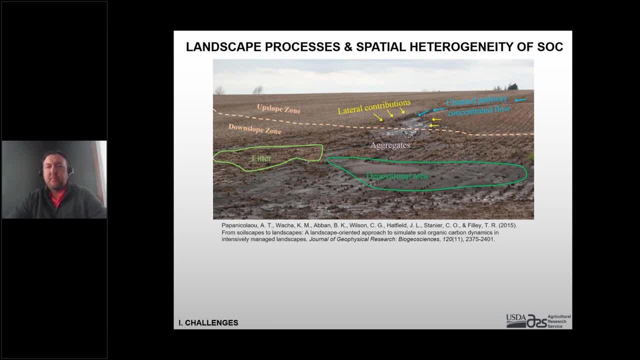 your fines and your your aggregates moving just all depending on what the flow conditions are, And you'll have stuff falling in and out of suspension in a lot of those channels and in the end you have a very heterogeneous landscape. So stuff depositing. 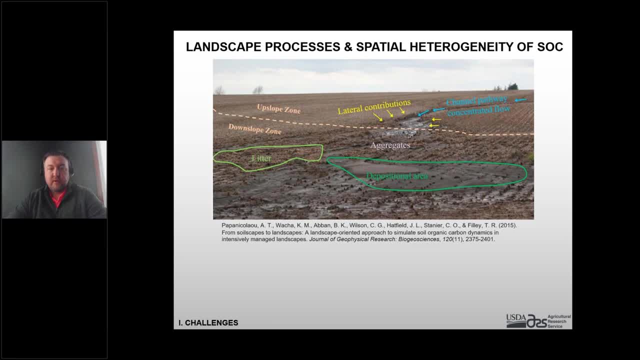 up and down the field. a lot of that can have impacts on moisture temperature which would impact your nutrient cycling. So a lot of the triggering processes from the erosion of the soil would be other cycles, biogeochemical cycling and just overall. 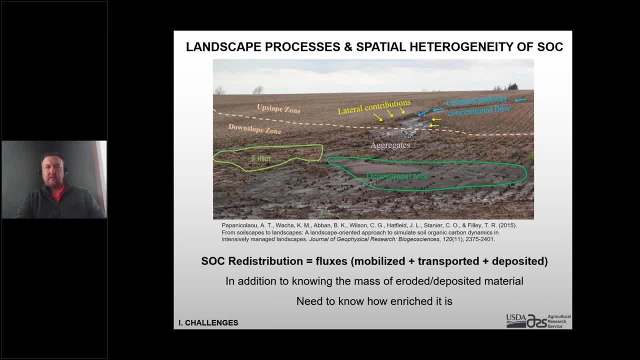 production which kind of throws a wrench in the whole carbon cycle. So soil, organic carbon redistribution. So redistribution is how, how that stuff's going to move across the landscape. A lot of it is is neglected. I'm thinking of 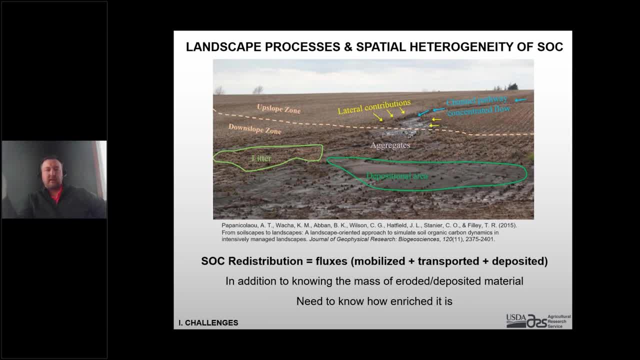 how it mobilizes, how it transports and how it becomes deposited. So one, how much of it is moving? how much of the material is moving? So like your erosion, your rate, or if you get like a mass of that. 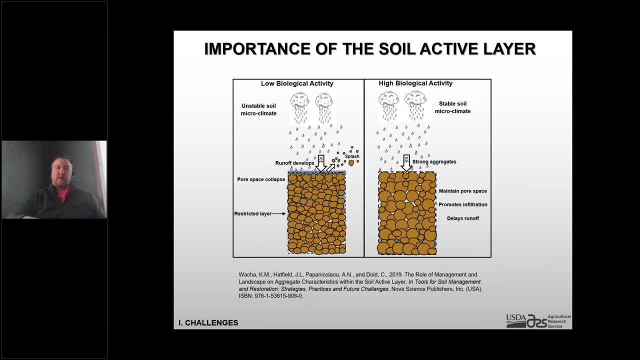 But also you need to go in and look and see how enriched that material is. So, knowing that that rainfall is going to become more intense. this how we treat our upper soil surface, which I like to call the sole active layer. 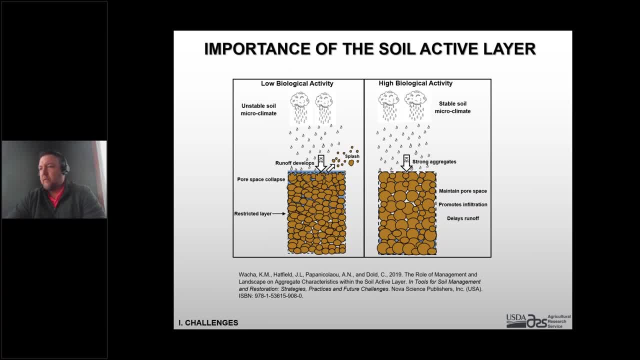 that's kind of the skin or the interface of the soil. So how you protect it with either a residue cover or, you know, your canopies, promoting stronger, resilient aggregates, increasing your microbial activity within the soil, to keep you know. 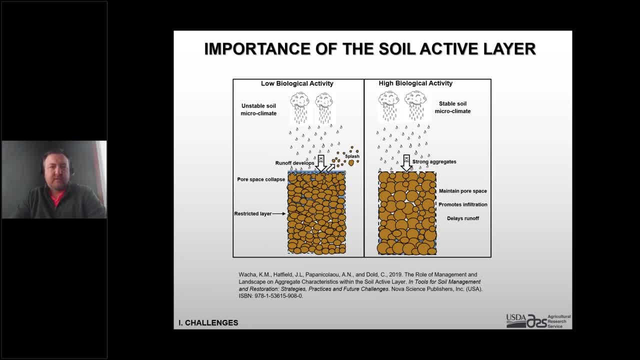 keep those things working and building aggregation processes are really going to have a big impact. So I'm showing here two different systems: a low biological activity and a high- And basically rainfall is coming down upon them- and the kinetic activity. 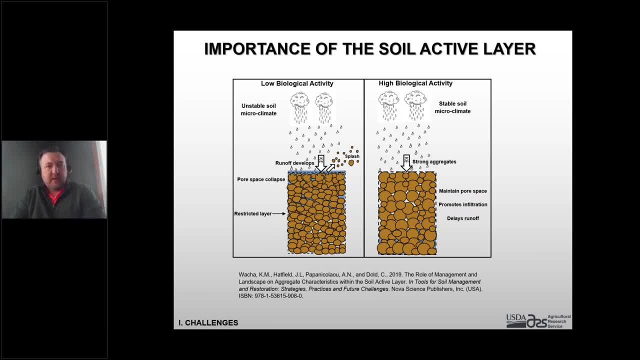 a lot of those aggregates within your soil structure there become weakened. The drops can collapse a lot of those pores as water starts to go in, A lot of the pores within there can restrict and confine off and cause like a restrictive layer which promotes. 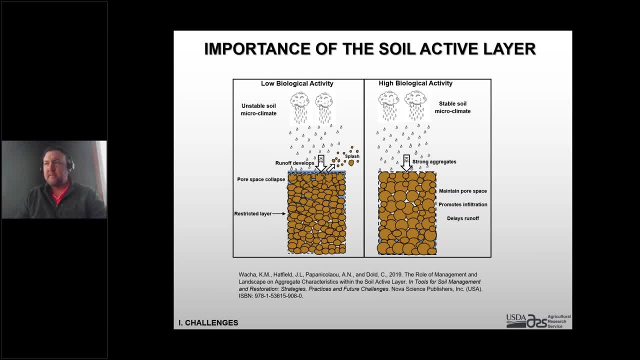 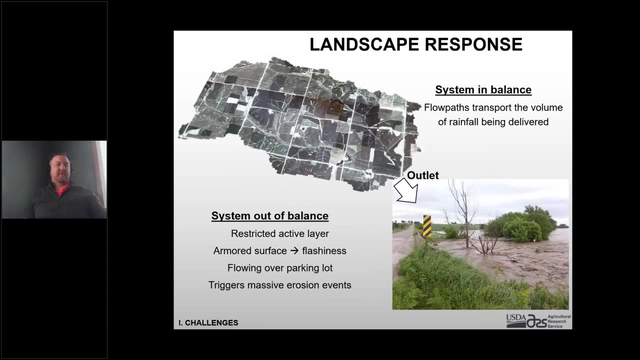 runoff to develop your splash and all the beginning processes, as I said about the erosion processes. Now you get into a higher biological activity, stronger, basically where it belongs. So understanding that we have the, that interface there, that soil active. 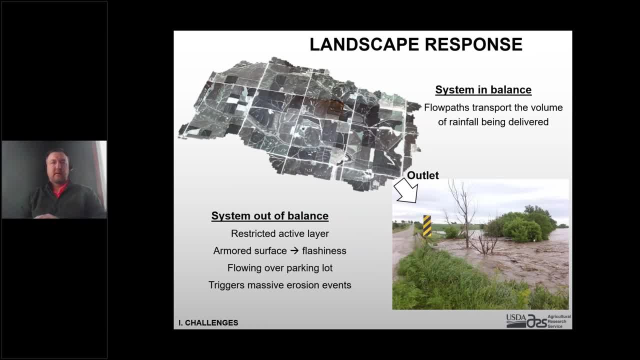 layer and that's just within a little soil column. we just looked. you know what would happen, you know, if you look at a landscape response. So what we see in that top left there, that's a like a little small catchment. 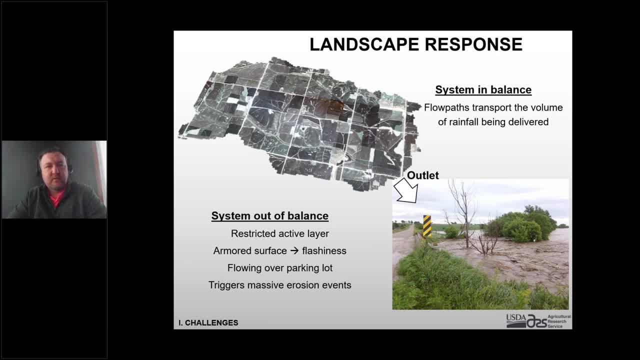 and it's kind of like the little drainage networks along there. lots of different fields and stuff are going to be supplying us. So if you think about a depth of water that would occur during rainfall and if you apply it to that, would it be this: 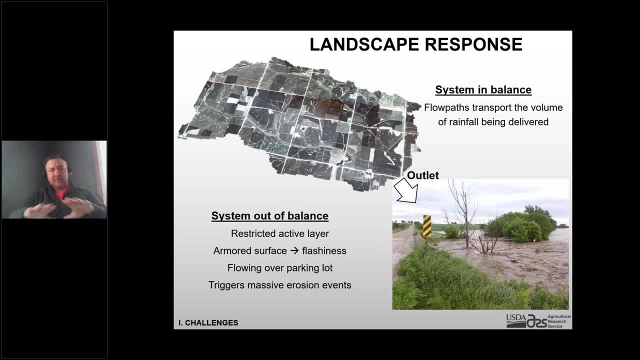 what's the system response? you know what's going in, what's going to cause a runoff depth, what's just going to cause shearing and different erosion processes to be able to transport material without that system. Assistive imbalance, all of those. 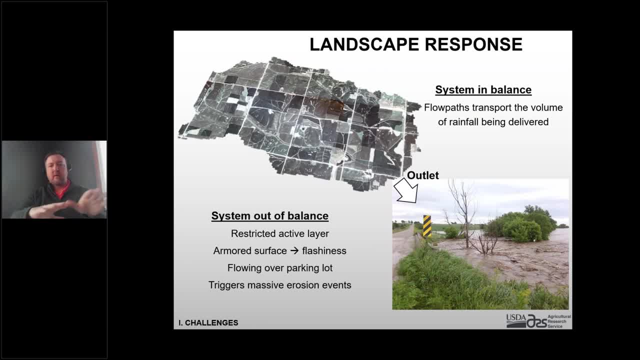 little flow paths are moving water efficiently. It can handle the incoming versus outcome, outgoing or, you know, hopefully like a very long timescale If a system's out of balance. what I showed on that last slide is that you could have restricted. 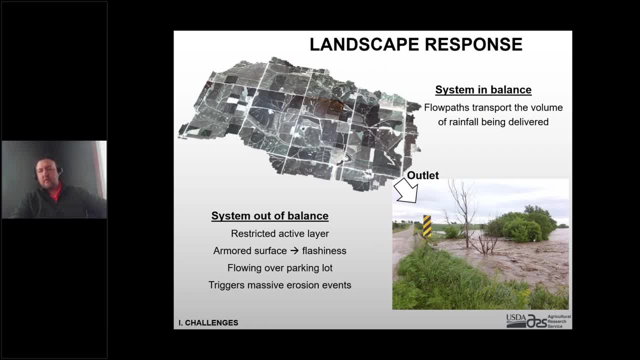 active layers, A lot of this from intensive tillage, different, you know, more conventional managements that just are not harboring your more resilient aggregates. So if those start to restrict, basically you could think of it as concrete. you could think of it. 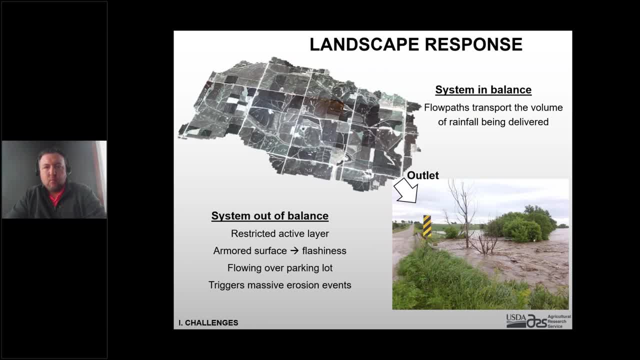 as a parking lot. so the rain's coming down and water's moving way too quick. it's not having the time to go within the soil, triggering these massive runoff events, triggering massive erosion events. The picture in the bottom right: this was around. 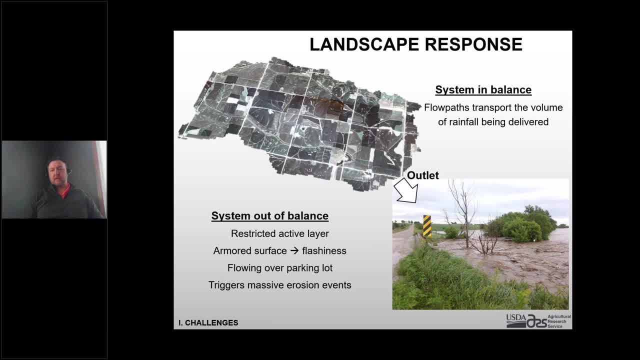 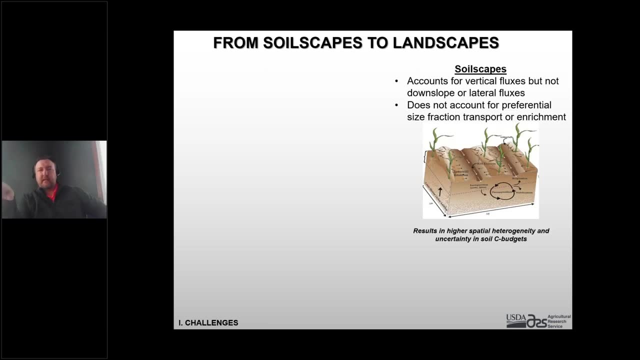 Iowa, 2009,, where we had one of these flashy, flashy floods come, And a lot of that is just due to an overwhelming amount of runoff, you know, supplied from all over the country. So moving from soilscapes to landscapes. 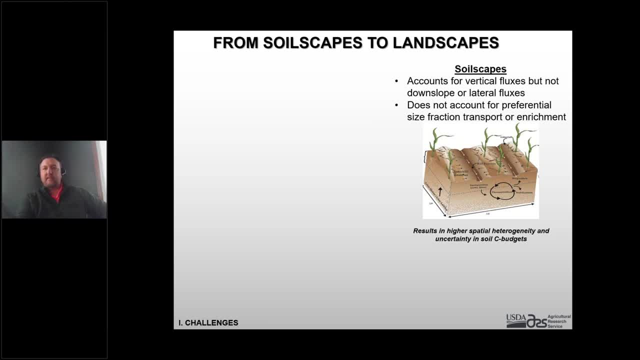 So, knowing how dynamic that whole landscape is and the spatial representation of properties and different managements that everybody's going to be using in there, it's important to move away from a soilscape which I like to think of as a it's a homogenous. 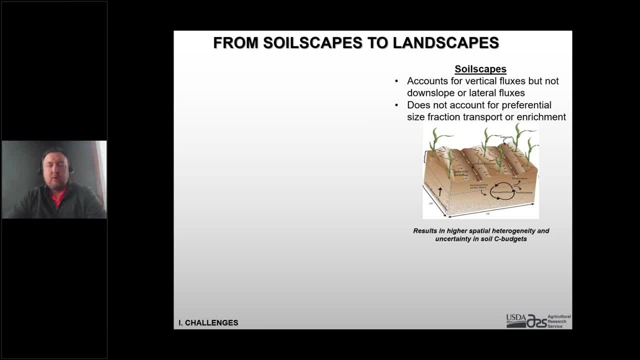 unit of land. this is representing the conditions that we're in right now. However, soilscapes: they do account for the vertical fluxes, So incoming sources of, you know, dead plant material comes in decomposition, cycling and respiration. 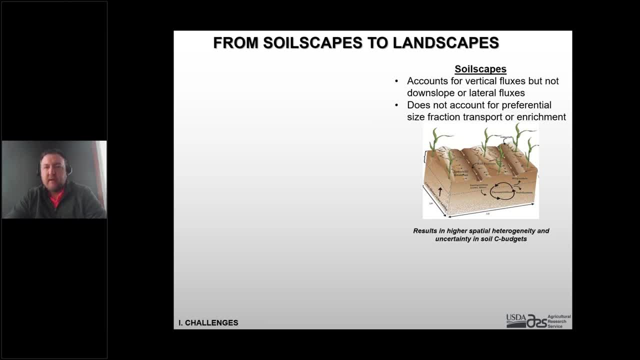 out, But then they do not account for what's coming in and out of them. So lateral and upslope, downslope transport, And this does not account for any of the things that we're seeing in propagating downslope, as you've seen. 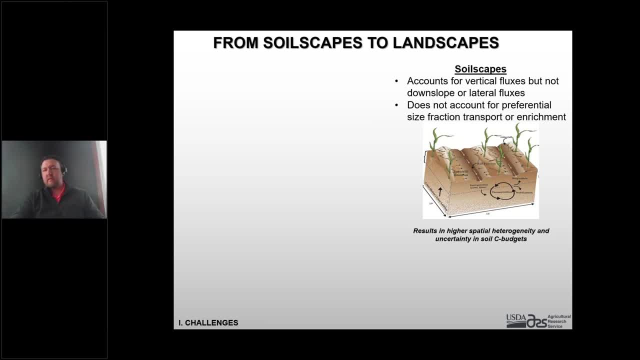 in some of those flow paths. What this can result in is, you know, high uncertainty and going out into a field- I mean, like I showed, there's going to be a lot of different spots in that field where you're going to have a lot. 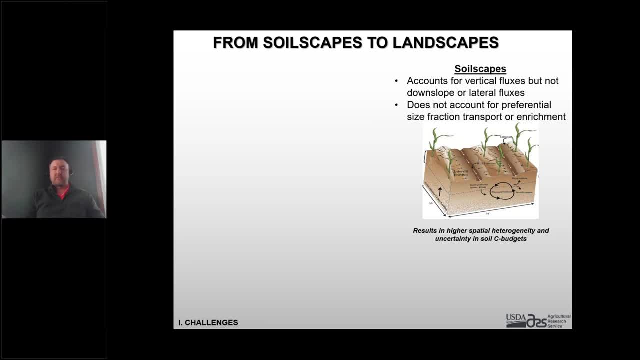 different carbon contents. A lot of that is because that movement and redistribution across the landscape. So you're going to see, just like a regular field there It looks pretty active on the landscape. You know, would you treat that whole system as just the? 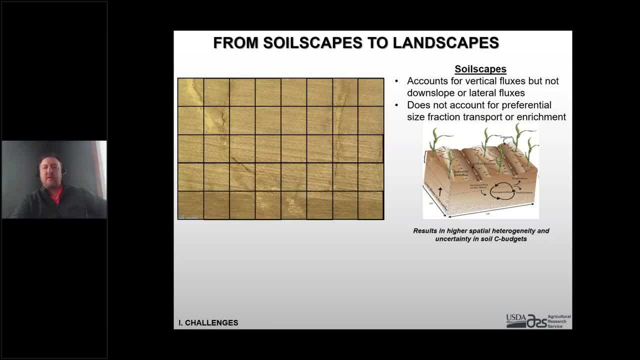 lateral fluxes in and out. It looks like there's going to be some changes there. So if you gridded that off and you treated each of those little squares as a separate little soil scape, you see that there's going to be. 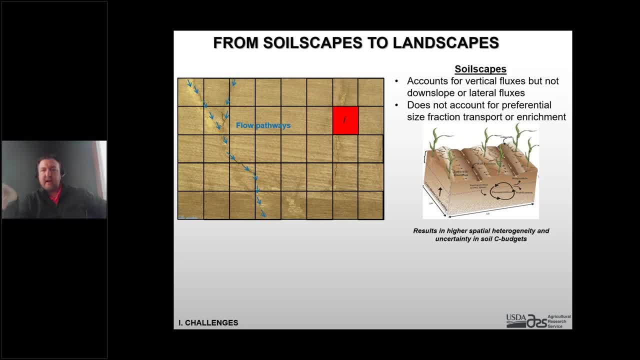 a lot of different inputs, outputs and transport along the downslope, That little section there, the red block- I think of that as that little soil scape over on the right And what you could do is you could account for those different inputs. 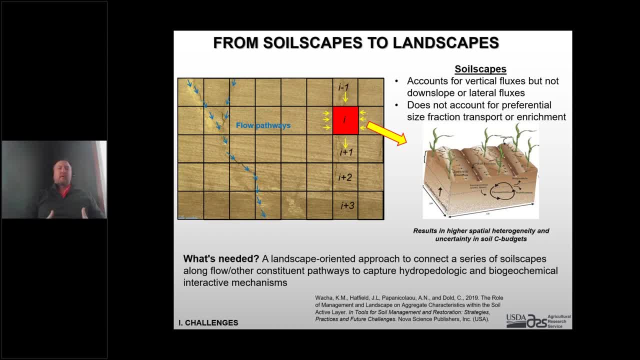 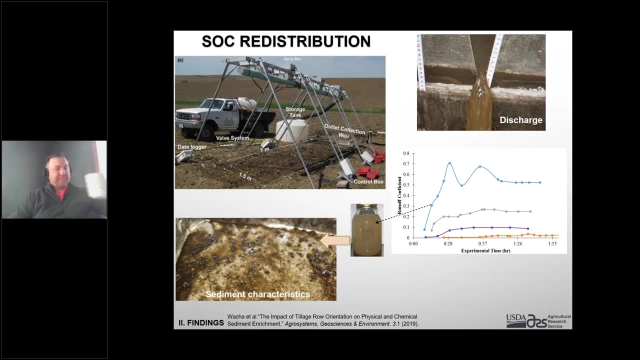 outputs and transport along the downslope to be able to capture those processes that are impacting a landscape. One second So soil, organic carbon redistribution. I'm going to show you just a couple some of the work I've done in some rainfall. 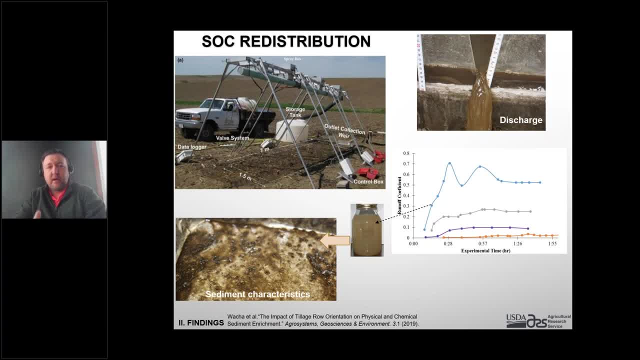 experiments in knowing kind of the process that I just described what I'm after. in some of these experimental designs I work with some rainfall simulators. on the top left This is kind of our experimental setup And basically we go out and rain on some. 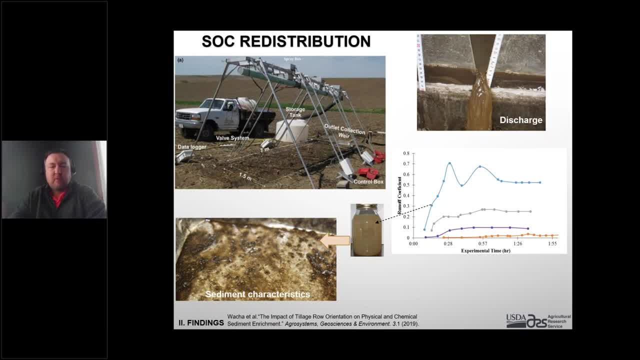 plots. We put a weir at the bottom And we'll look at kind of the time series and the response of runoff And basically within that time series we're going to look at different intensities we can use, We go around to different 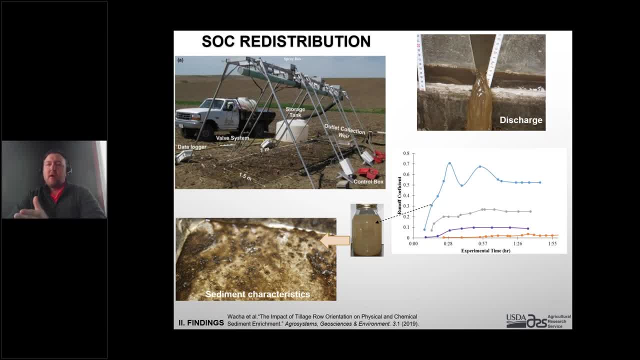 sections of there. That's kind of if you go back on the slide before and one of those little gridded sections there. we're just trying to understand what's going on in that section. So we're going to look at the. 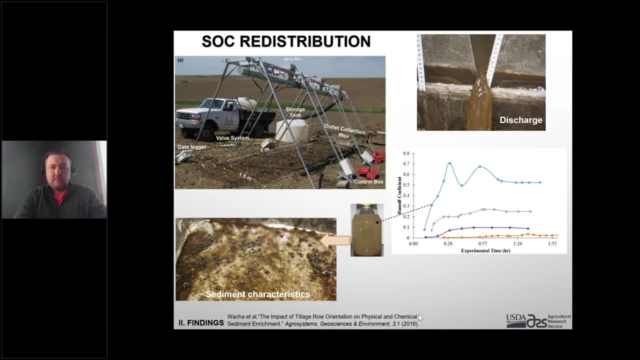 runoff coefficient. and the runoff coefficient is going to be the depth of precipitation being applied to the runoff that's being coming off of it compared to that depth of rainfall. So a value of one would be: whatever's raining on is running off Very low. 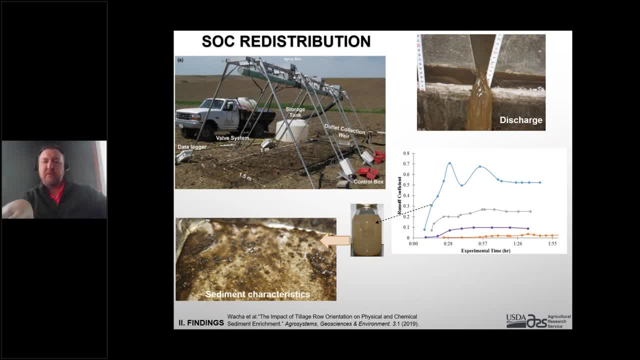 runoff coefficients means a lot of it's going into the soil. So not paying attention to exactly what those are, I'm just showing you kind of like the trends. you know, capturing that time is not just, again, the primary stuff. you have aggregates. 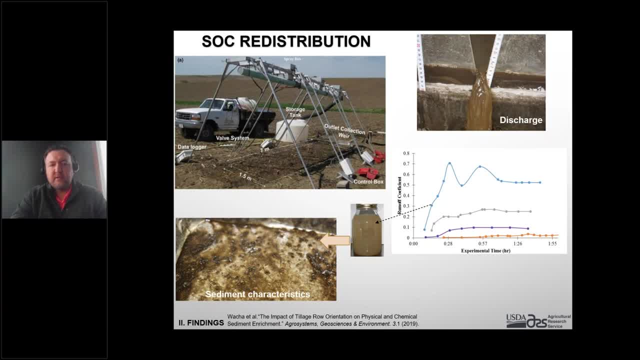 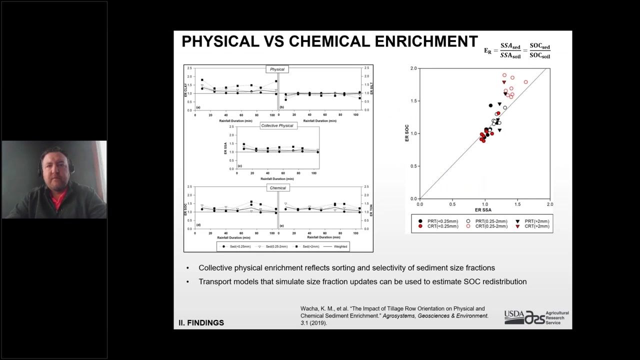 and different size fractions, moving along there and then looking within those size fractions and understanding you know the whole dynamics of aggregates and you know what they're encapsulating. by not accounting for those, you can be way under over. you know estimating your carbon content and then 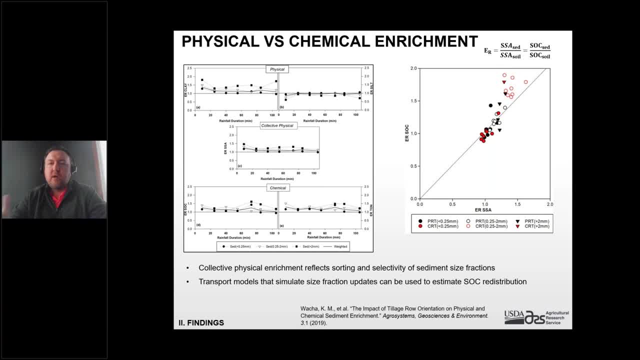 you can see what's happening in the soil. So what I was working on developing was: can I relate that material coming off there, can I get an idea of those size fractions and be able to relate that to a carbon and to be able to? 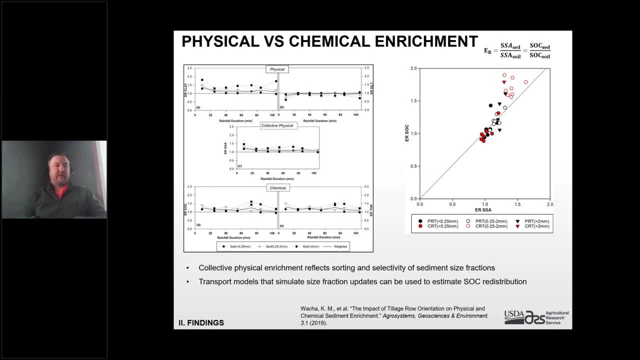 simulate the different movement of those fractions with different events and then be able to tie that back in and have an estimate of your losses of carbon. you know moving and transported during different intensities. So on the left over here there's three different sections. 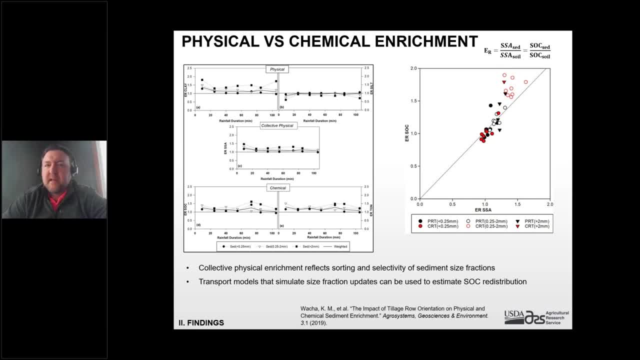 So, going back, what kind of this, what would be in the sediment and that can be broken apart into through different sieving techniques, different size fractions within there? For this one, I have three shown. it's on the bottom there it's less than 0.25. 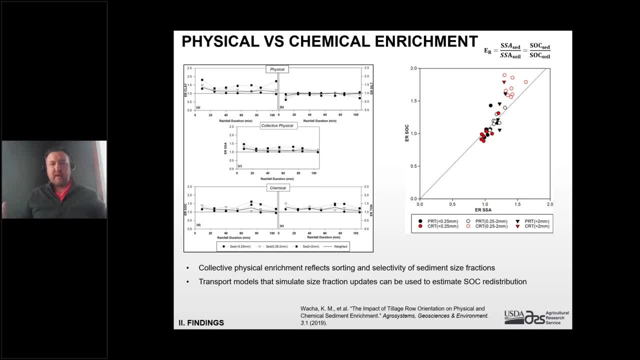 millimeter, 0.25 to two inch, and again you can estimate what's in that section. So on the top left you've got your Levine and then on the bottom you've got your silicon at the bottom and then you've got your soil. 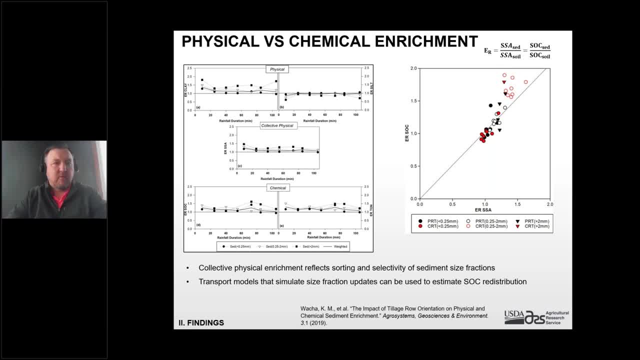 in than what was there. you'd have a more enriched. so values over one are going to show that you know a lot more of your fines are moving within those cases and it tells a lot about, um, the characteristics of a certain rainfall event, like right away you have some stripping of the, the aggregates and 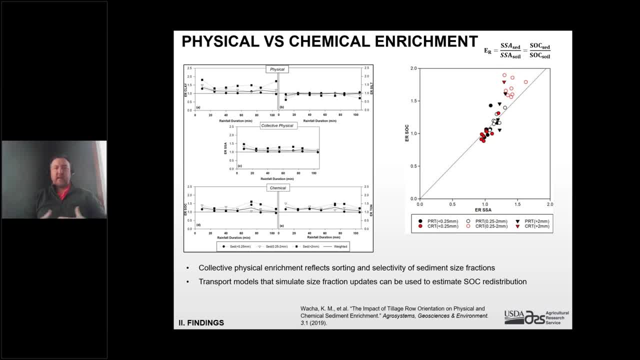 peeling off um the outsides of it and then, as you go on, it might, you know, disrupt the whole aggregates and then large events. you may see that everything moving is very similar to um the type of material that's there. so values usually go towards the value of one or unity. 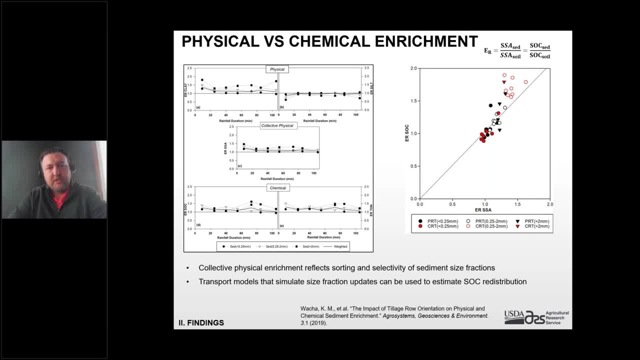 um. so taking those you can, you can make a relation between the texture and then the bottom there, the chemical which i um, the carbon contents. so on the on the right hand side, what i found was there's a good agreement. it's been pretty well established- literature as well- that you know your finer. 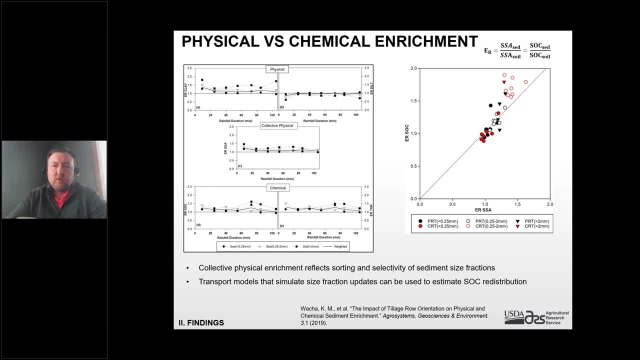 particles, or your, your particle sizes, can adhere carbon. so making that relation between, um, the specific surface area of your sediment, with your carbon and nitrogen, that you can be able to use an enrichment ratio to be able to describe not only the amount of sediment moving but um what, what's within it, or you know how enrich and you know carbon transport. 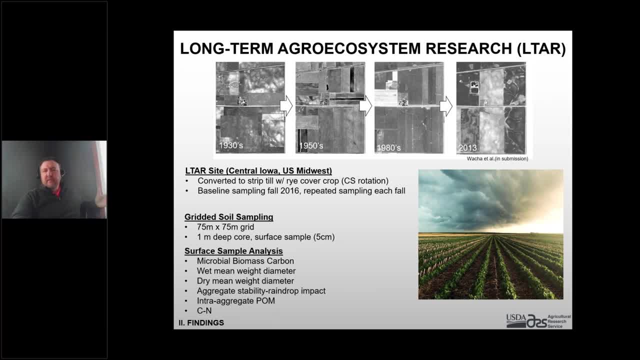 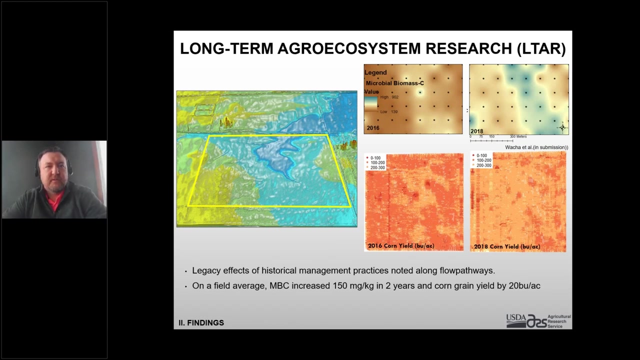 and some of this can be applied to the fields and understanding you know, different ferritic and soil nature management um. how's the impact on the different drainage networks within their transport? how does that affect the spatial um distribution of different properties? i'm just looking my time here. i'm going to hammer through here, all right, so this is one of our LTR. 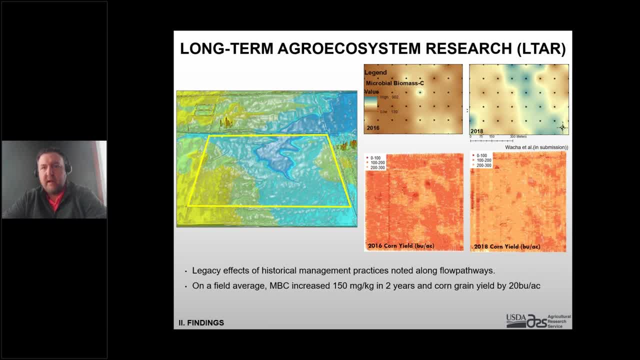 sites, a long-term ag site. i got it boxed off over there with that yellow and just looking some changes in management and seeing um- you know how active these term is- um, as we kind of move our or the landscape has been in within um just a two-year window. so what? the system in the in the 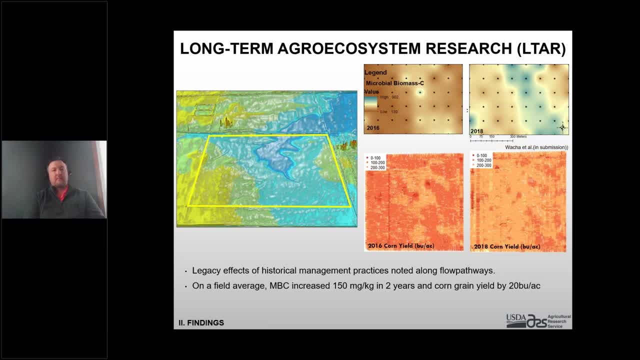 first year was was, it's very conventional, tilled um, you know no cover crops. it's just a corn soybean system. two years later, with cover crops and you know no till, there's been a dramatic response, whoops. so looking at those little arrows there, you can see the dynamic flow paths within the 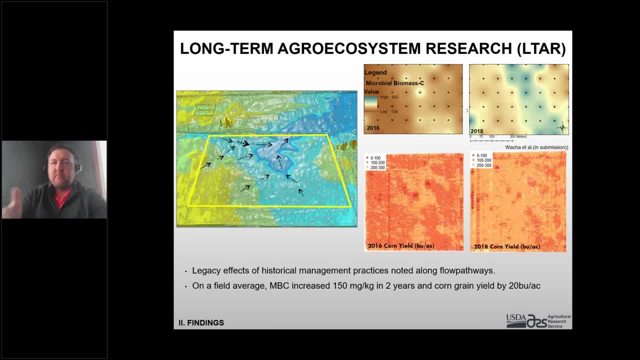 within the network. they're kind of showing how the water is going to move and you see a lot of the properties there kind of follow that same trend. so the upper right you see microbial biomass within the, within the soil, huge increase almost, um, i think it's 30 or more. 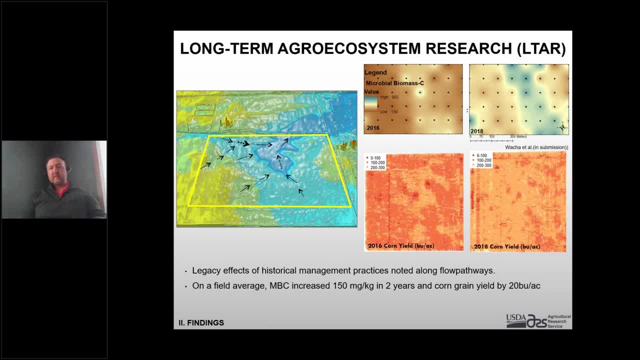 within the two years. so you're, you're, you're protecting that sole surface, especially within that, that upper, upper layer. you're promoting microbial activity, more aggregation, more ということ, and um, the, the uh, again that, the, the, the. this is what we're looking at is actually 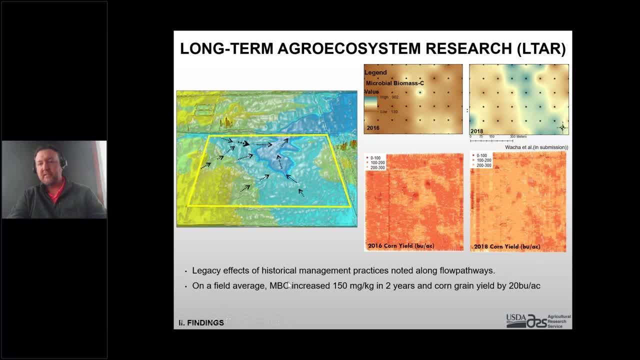 a split. you know it's. it's very drought resistant, it's a fairly fine and, uh, more monolithic um group of crop crops and the other things you'll notice within the study is that this is this is that this is not the same area as the front and this is um. 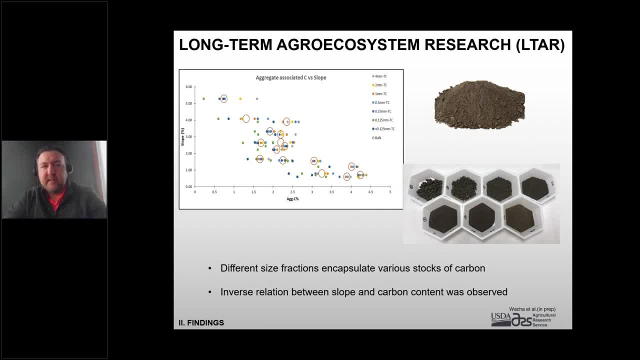 the same area as the front. yeah, so we're trying to figure out what happens when we draw more of a row along a massa here, with a more monotonous growth of the crop over a? uh, in the center of the field and, you can see, with a more homogeneous growth of the crop over a number of years, there's some gaps in the 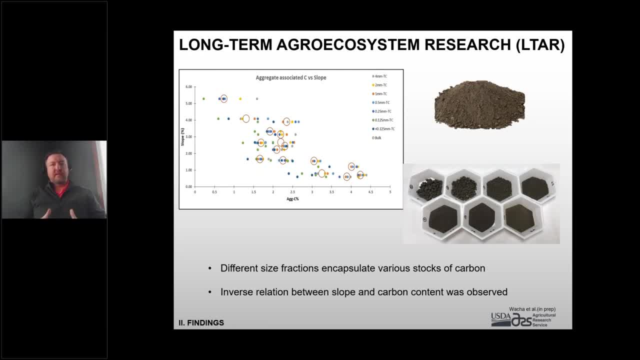 these aggregates, you can see there's just a lot of different contents within these different size fractions and how how that relates to slopes. there's a good trend in there of inverse proportional to slopes. so if you look at this kind of a line of these here and you look at what 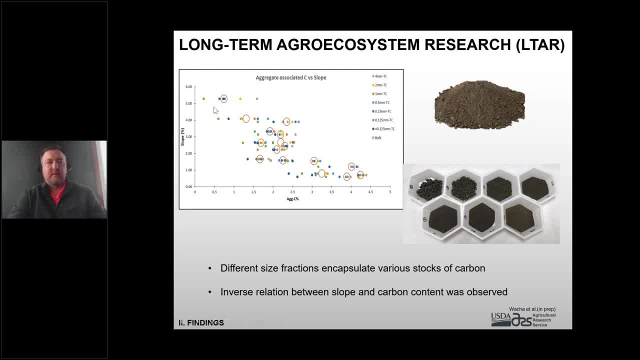 carbon content is in these different size fractions. you could see that it's a pretty good. you know range and understanding the importance of accounting for those aggregates within you do in your, in your redistribution, and um accounting for that within um soc. you know transport, so the the circles on there represent kind of that weighted you know. if you took the whole sample. 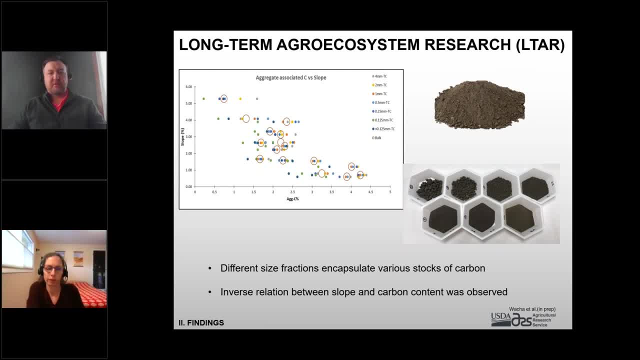 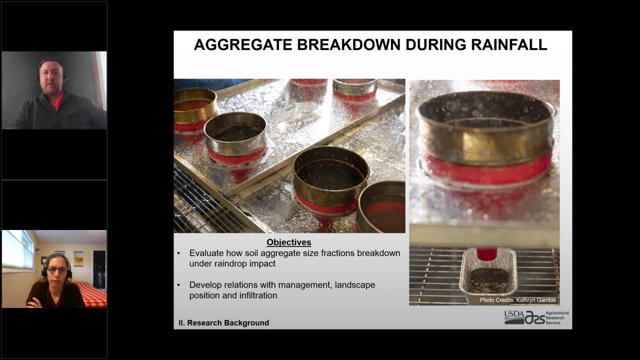 and you know, combustion or whatever you burn it, this is what the carbon content would be, but the importance of understanding the sizes and the distribution of them and moving to be able to better account for transport within here and again. this could be applied again to the, to the rainfall, the breakdown you can see kind of a nice little. 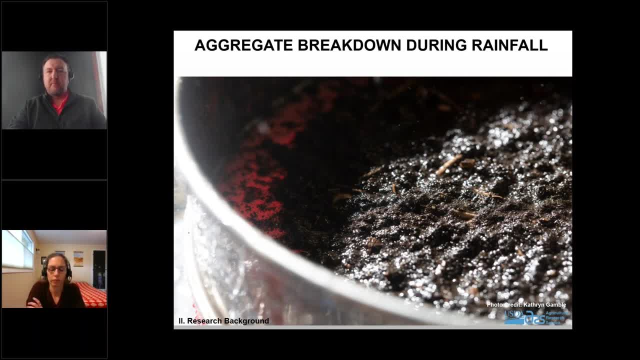 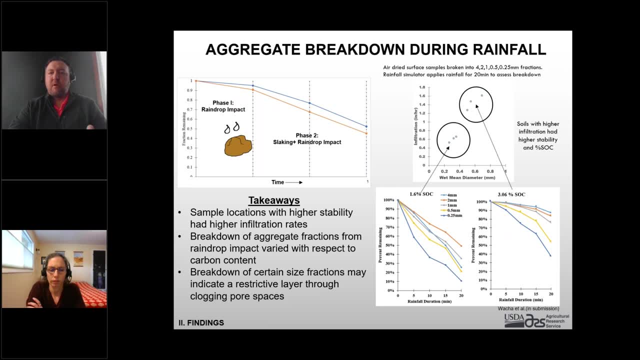 snapshot there of some of those organics within the soil being broken out and, you know, dislodged during during storm events and what those can have as as impacts then on on allowing water to move in and out of the out of the soil profile which is going to be at that direct interface for higher rainfall events. 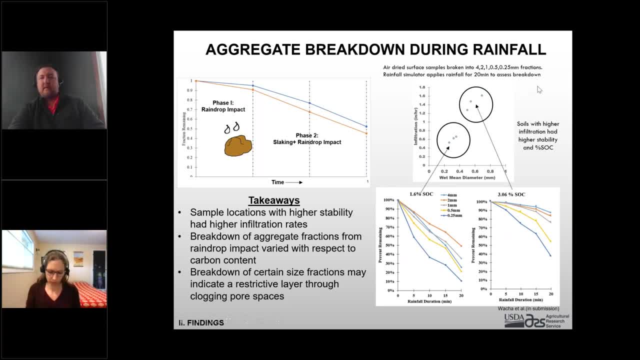 which is going to be at that direct interface for a lot of the more dramatic precipitation events. i'm going to show this last thing here and then i'm going to wrap it. you know, some of the experiments i'm running is just isolating those aggregates and seeing how. 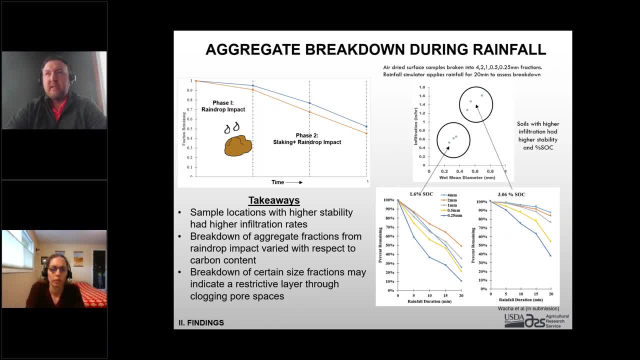 they break down in time and kind of what's? what's the response there? because i believe that we could take our aggregates and it can provide kind of an x-ray of what would happen in your field. so if you go out and perform a graded sampling and you know the characteristics of weak aggregates, 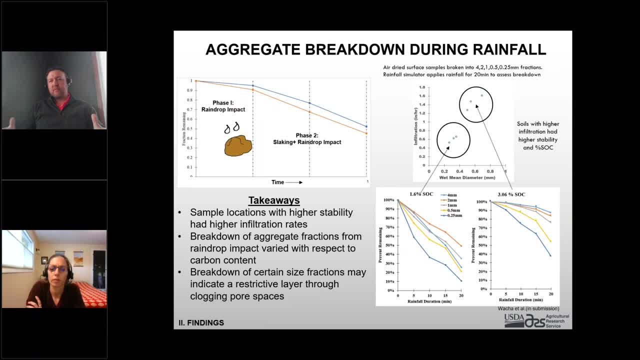 compared to strong or what's in them or what's the distribution of fractions. you could kind of uncover some patterns within your landscape and understand that if you did apply a depth of water, some areas it's gonna go in, some are gonna be very restrictive. 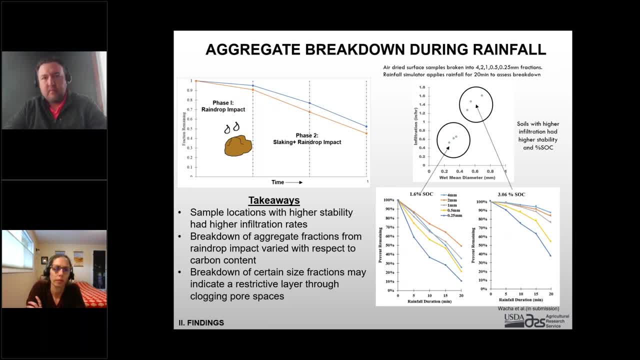 You can kind of uncover your flow path networks, understand why you have different areas in your field that are struggling to get your yields up that have low carbon content. It's because it's restricted with infiltrations. You got weak aggregates, collapsed, poor networks. 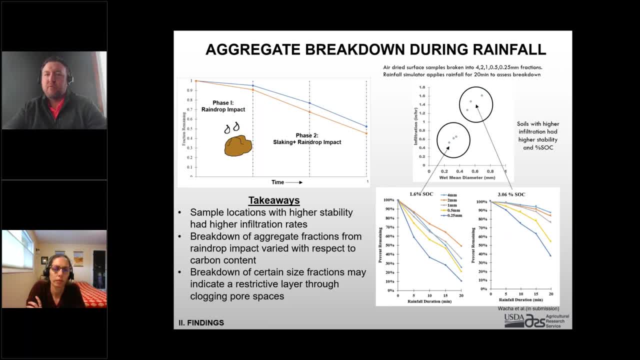 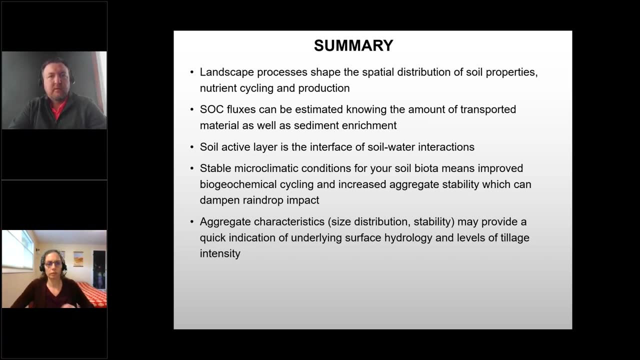 And then just to be able to bring that in kind of a systems approach to be able to better estimate kind of your accounting for your carbon redistributions in the whole system. So summary, landscape processes are called and are the most important And in the case of landscape processes, 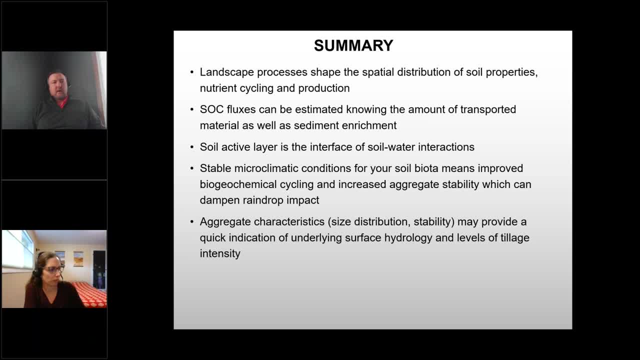 they're called structural. they're the most important, because they're the most important for how you're doing your work, how you're doing your production, the way you're doing the production, what you're doing the production and how you're doing the production. 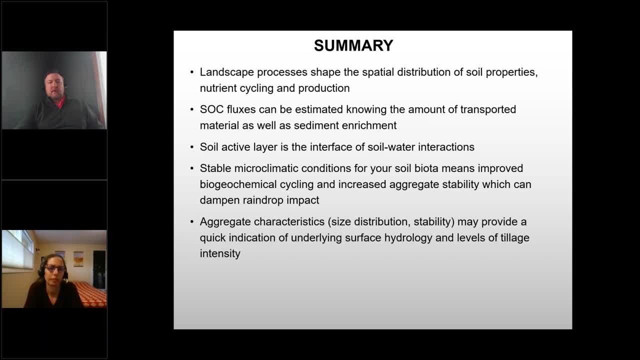 And so what does that mean? Well, it's a very basic question. If you're using a lot of soil in your system, you're not gonna get a lot of soil. You're gonna get soil in your environment, and it's just gonna be a little bit more difficult. 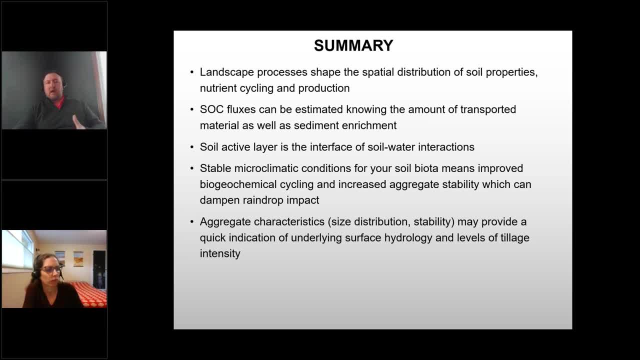 to be able to estimate some of these fluxes, we need to know not only what, how much of the material is moving, but how enriched it is, so accounting for those size, fractions and what what's, what's the characteristics of them as they move across the landscape. 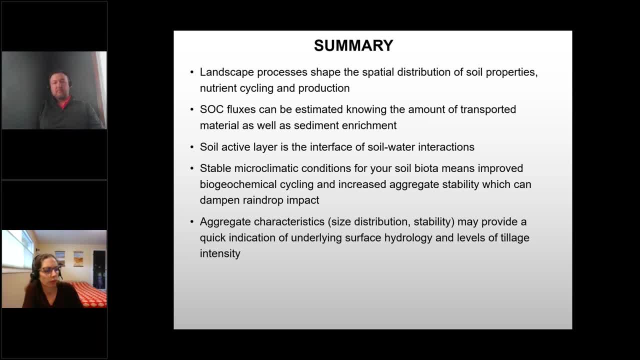 and to treat our sole active layer as a very important piece in all this, because it is that interface of the soil, water interactions to be able to build resiliency towards whatever weather change we see coming. and within that, that active layer, if we promote a stable microclimate. 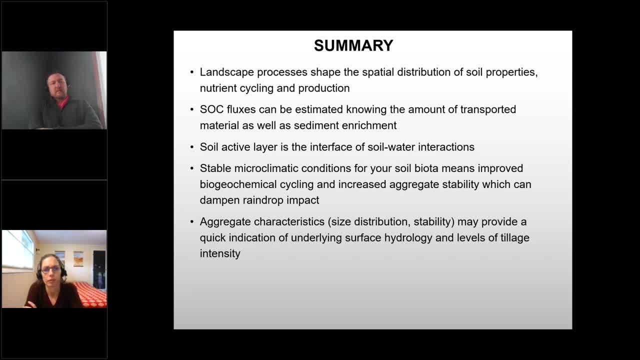 so something that's not getting flushed out all the time from you know, your rainfall events and collapsing all those pores where they live in. in there, they'll promote, you know, better biology, chemical cycling, stronger aggregates to be able to further build resiliency and, lastly, 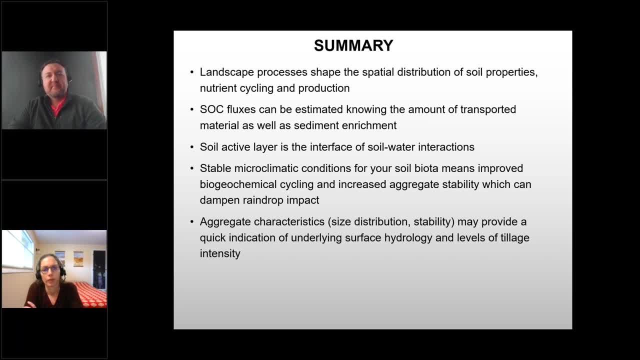 if you can't get out and run rainfall experiments and different things within different parts of your fields, looking at your aggregates, i think is is you could slap that out x-ray like if you're a doctor and say: okay, well, here's your aggregates. this tells me your tillage intensity is this, you know so. 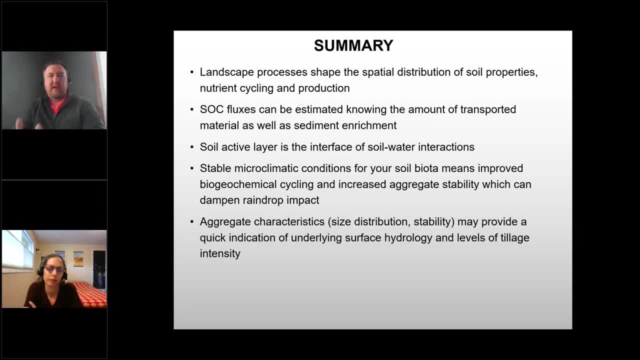 it shifts it here you know the distributions of that will tell you kind of a an inference of how much time you would have also, um, in a rainfall event. you know when there'd be a collapsing within those poor networks. so all these things could be helped to kind of better understand the processes involved and to be able to accurately provide. 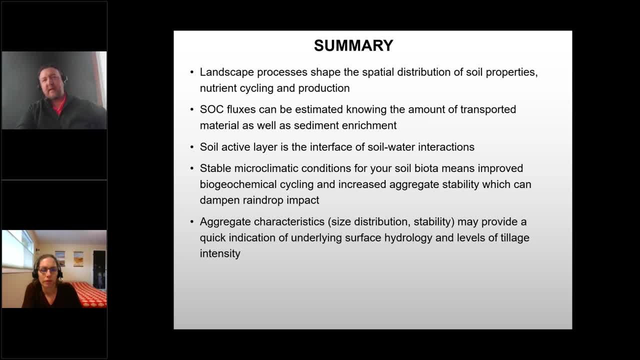 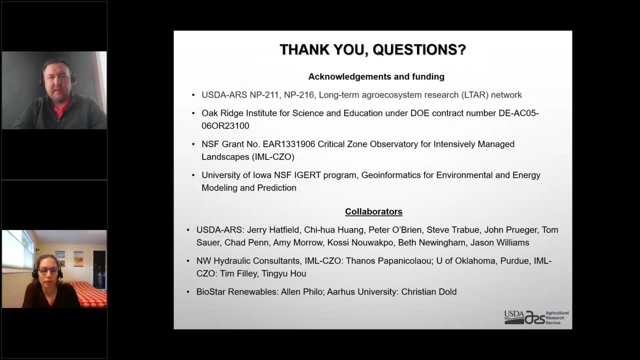 better estimates of carbon budgets by accounting for the redistribution. so with that i thank everyone and i'm glad to answer any questions. here's some of the acknowledgements of funding and different collaborators throughout some of these projects and it's really great to be able to continue international practice to make sure that we 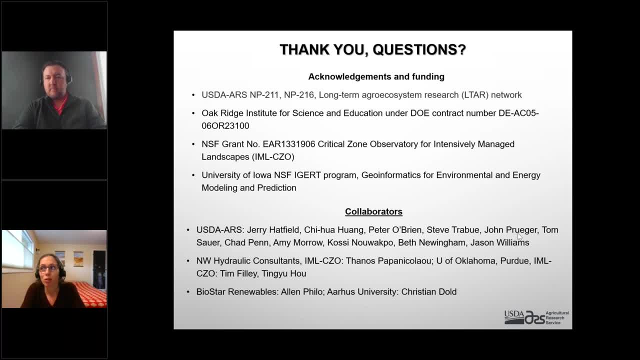 are gemeinsam and working together to figure out what we are and how we are going to build a sustainable and sustainable environment. so thank you so much for sharing and i look forward to your future conversations with you. again, thank you so much for having me. thank you, thank you. 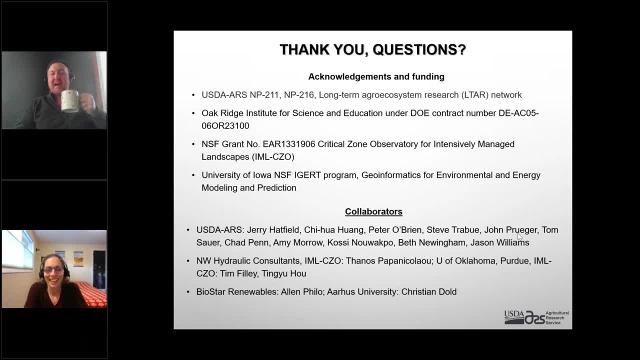 thank you so much for watching this. um. our next question is about: will there be a canary in the Yeah? so I'll just ask a couple questions. So I was saying that in one of our talks last year, Christine Morgan was talking about carbon sampling technologies And she made the point that, although 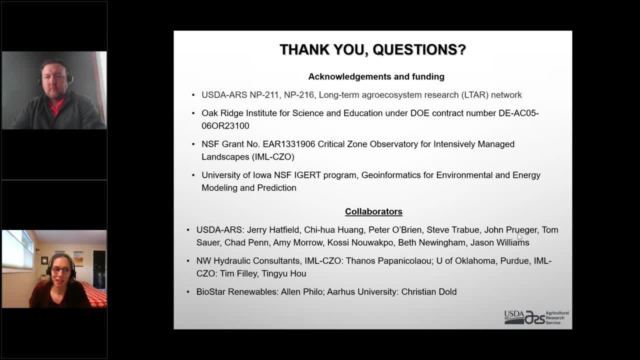 carbon distribution is highly heterogeneous on the landscape. it's structured And that gives us some hope for strategic stratified sampling protocols to be able to monitor carbon changes over time, And I think a lot of the work that you just presented gives us very nice mechanistic. 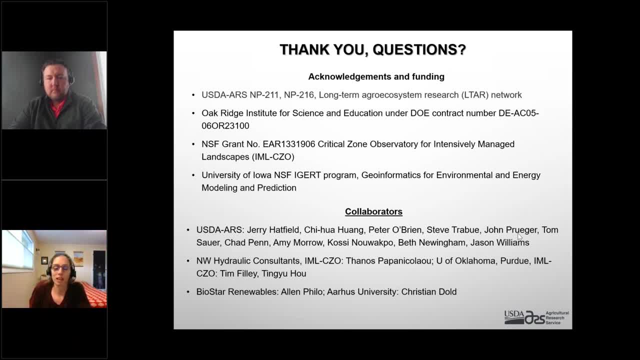 framework for understanding where carbon goes and how it can mechanistically potentially be modeled eventually. So I guess my question is: if you were to pick certain processes that would be a priority for including in carbon models, what would you pick? I would like to bring in, I'm trying to bring in, I want to bring in the aggregate. 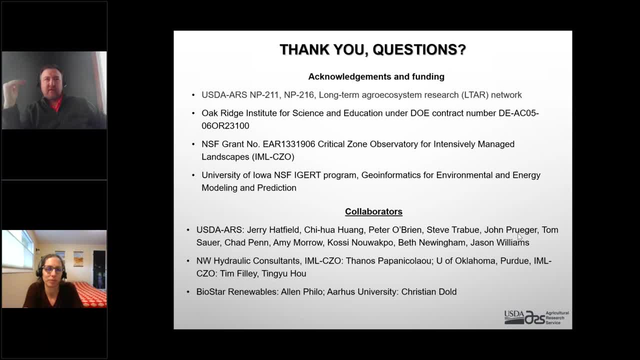 stability term as kind of the interface for the rainfall being applied to the soil. So usually they don't use an energy approach. It's traditional flow equation. So whenever your depth and everything's steady state model, But I think that there's a lot missing by the energy being. 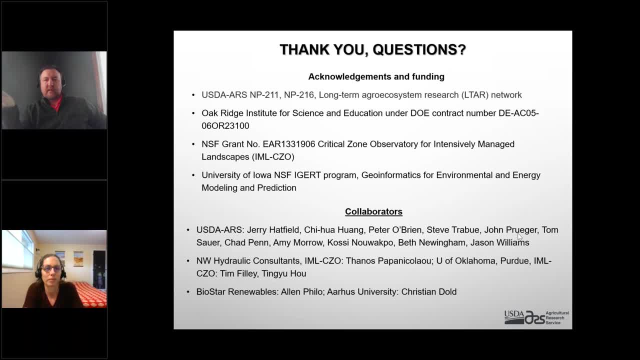 applied and the response of the aggregates. You know they think that it's very misrepresentative of when it's going to actually. you know runoff will be triggered and so forth. But so how you treat your aggregates, I think it's a really good holistic way to cover a lot of ground because I think it can reflect 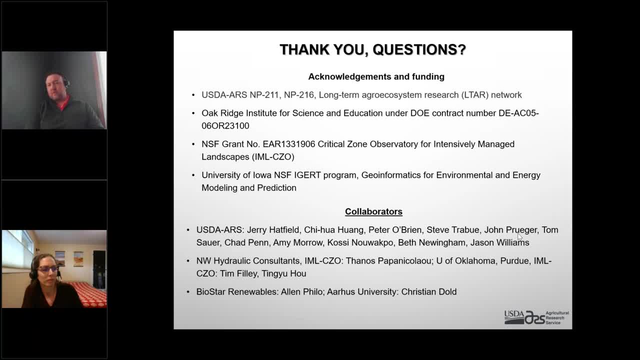 infiltration rates and also resilience to those drops and you know kind of your Even for respirations and so forth. So it's kind of a way to tell a lot of things with not that much work to get that information. So I think it could be implemented very easily in a lot of different scales and so forth. People should 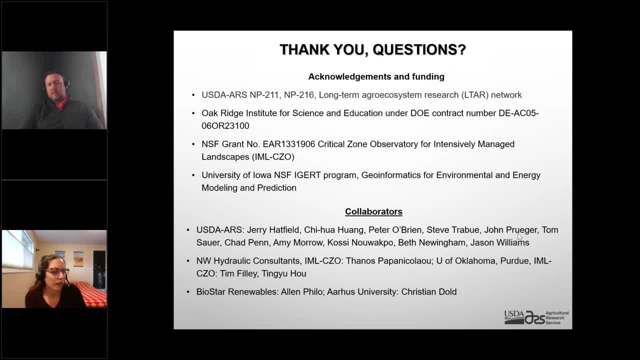 have that data. Okay, And then the last question I'll ask you is: do you take the underlying stratigraphy into account, when I guess this is in the context of if you've been doing a lot of work with the surface carbon movement? if you were to model surface carbon movement, do you take the underlying 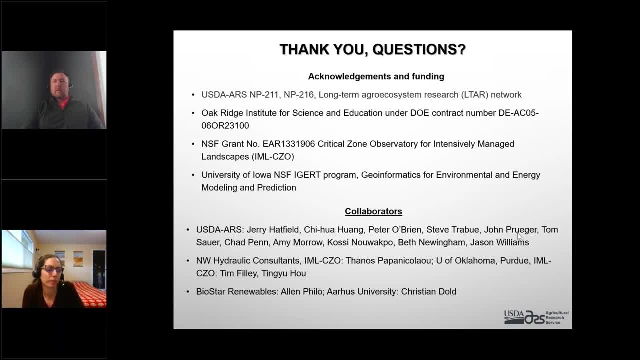 stratigraphy into account as well. You know, like there's a parent layer. I guess, like for some of those frameworks it's super, I mean deep layer or anything you start getting below the surface is. I guess that's funny: You scratch below the surface. 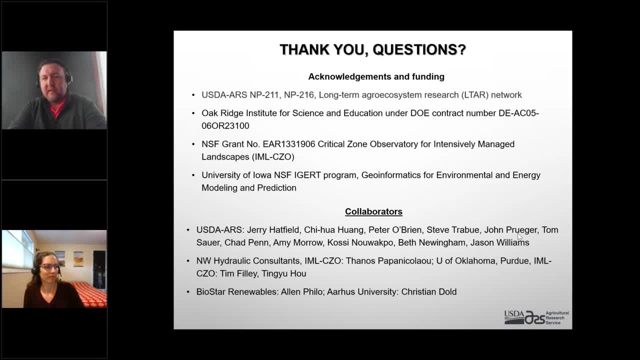 But no, it needs to be better accounted and connected in there, And so it's just a way to kind of make sure that the surface has a more robust, more robust surface in the environment, and then it's a much more, Much more emphasis to connect subsurface with surface. But a lot of this I presented was just 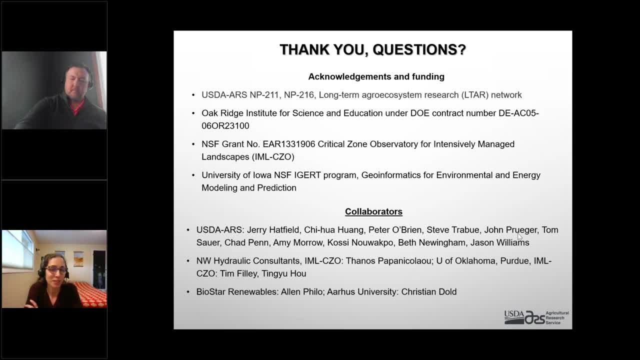 that interface, knowing what's coming, then that's kind of where I was at. Okay, great, So we have gotten to an hour, so I got to let people go, But I just want to thank both of our speakers. so much again for joining us. 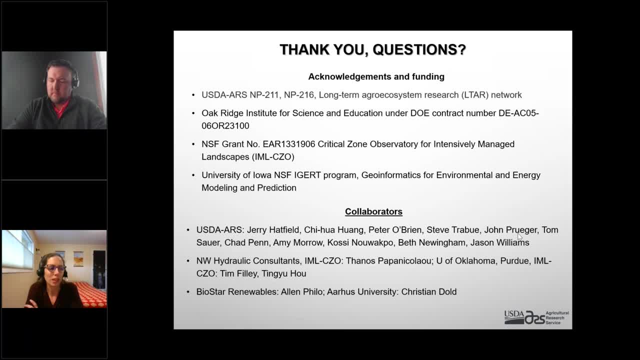 us next month, in March, where we'll be taking up the issue of carbon saturation and how that affects sequestration potential. So thank you everyone.